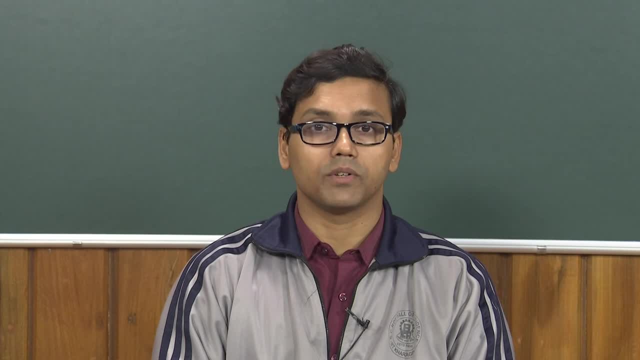 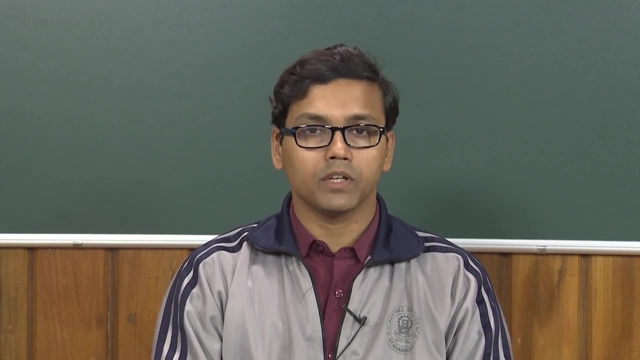 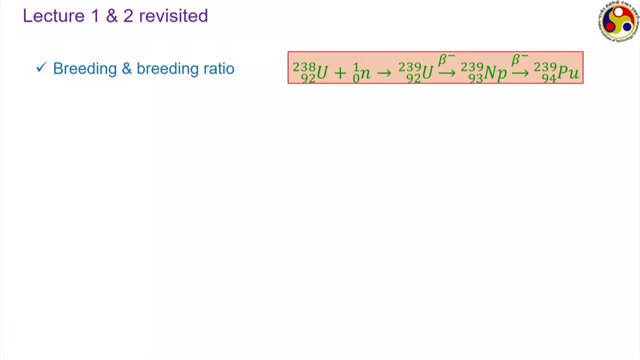 the difference between of a breeder reactor with a conventional thermal reactor. Just to have a quick recap: in the previous two lectures we have discussed about the concept of breeding and also the breeding ratio. Now we know that the term breeding basically refers to a reaction like this, where a fertile nucleus absorbs a neutron and that goes through. 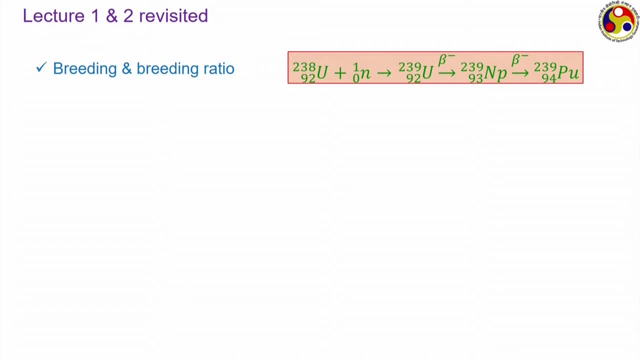 successive decay processes. In fact I should not say all the breeding reaction involves such kind of decay, but the common reactions, like in those involving uranium 238 or thorium 232, is always. in this cases you will find such kind of decay That is, one neutron absorption step followed by two successive steps of beta decay leading. to the final product of plutonium 239 in this case, And when it starts with uranium, thorium 232, then, after absorption of the neutron, we get thorium 233, which goes through two successive steps of beta decay to produce uranium 233.. But there can be other kinds. of beta, sorry, other kinds of breeding reactions as well, which which are direct, like plutonium 238.. So plutonium 238 can absorb a neutron to produce plutonium 239 or, more commonly, plutonium 240 can absorbs a neutron to produce plutonium 241, which such kind of direct single step. 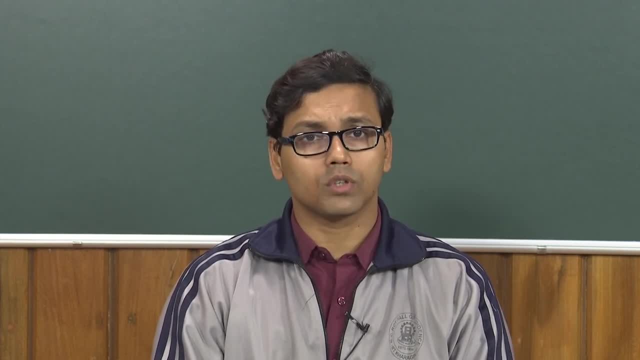 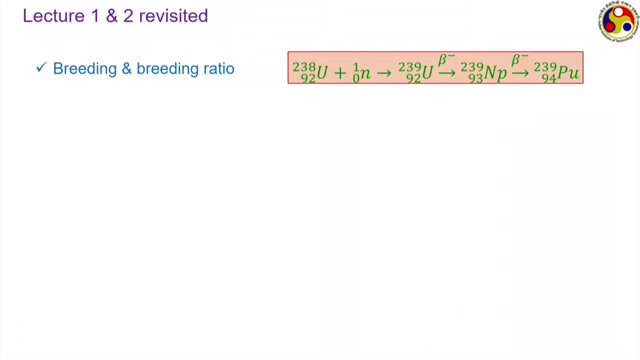 breeding reaction is also possible, But generally the two most common kind of breeding reaction that you will find in industries: one referred to, the one that is shown here, uranium 238, absorbing a neutron to produce plutonium 239. And the other one which goes through two: 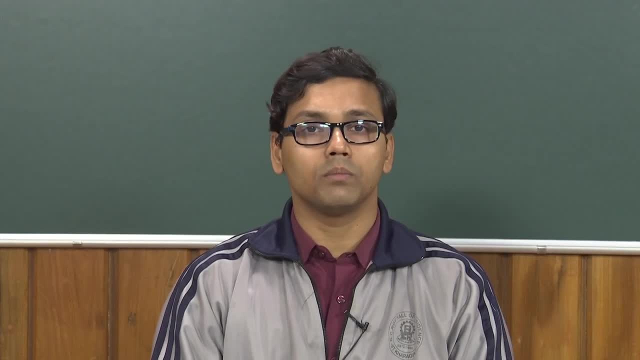 successive steps of beta decay, which is of which is of increasing popularity, where thorium 232 absorbs a neutron to produce uranium 233.. As I have already discussed that thorium reserve in the world is at least three times more compared to uranium And therefore, and its primary isotope is also the uranium 232, just like uranium 238 in case of uranium, And therefore several countries are looking to build their future plan of action in case of nuclear power production based upon thorium, which involves India as well, Like Indian nuclear power program. 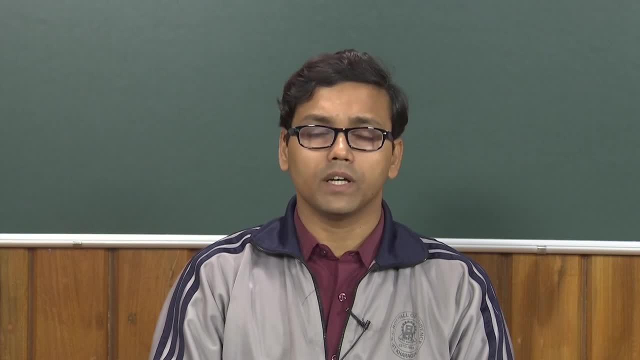 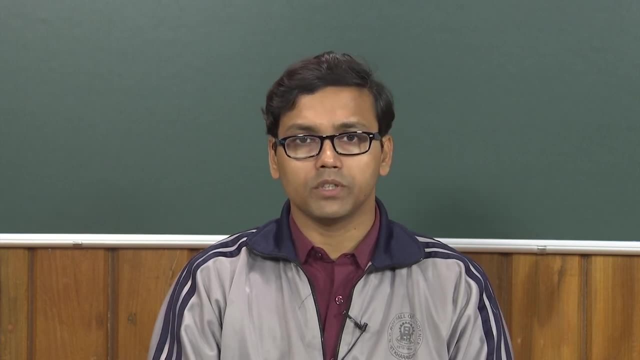 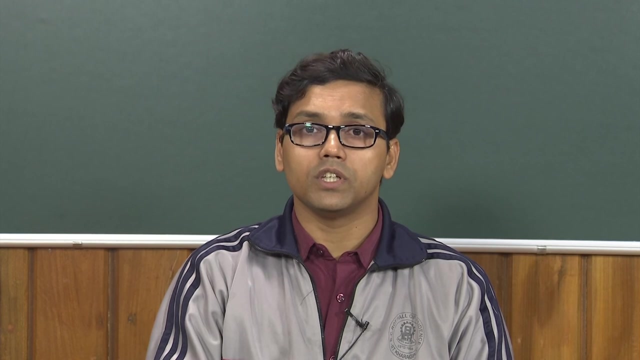 has a big dependence on thorium. India has quite a small stock of uranium but very large stock of thorium And therefore we shall be talking about later on in the next module where you will find that the thorium 232 plays a big role in Indian nuclear power program. 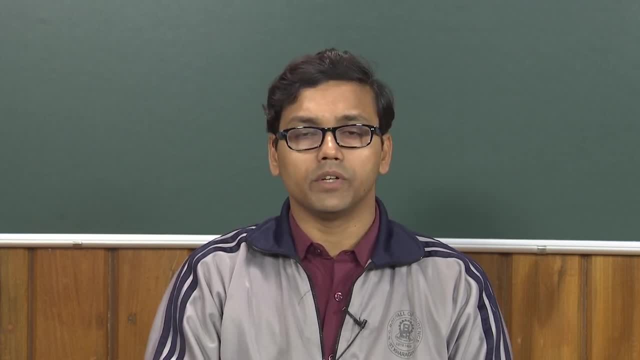 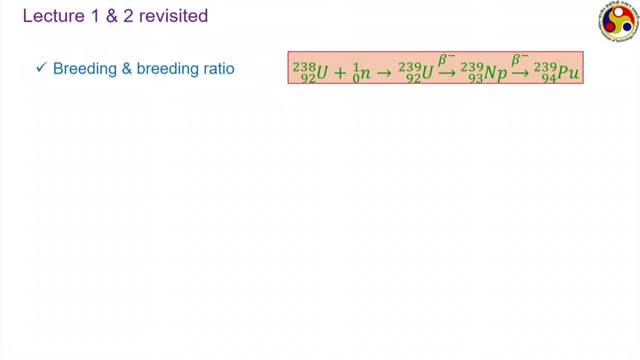 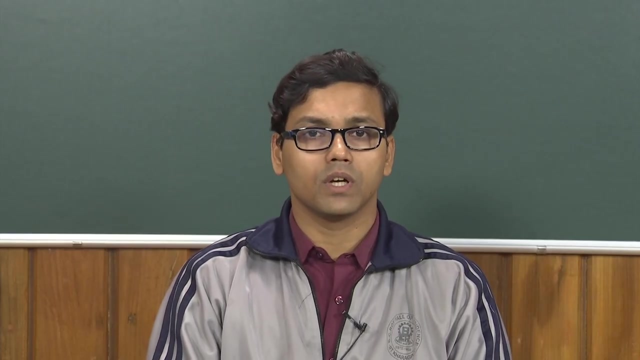 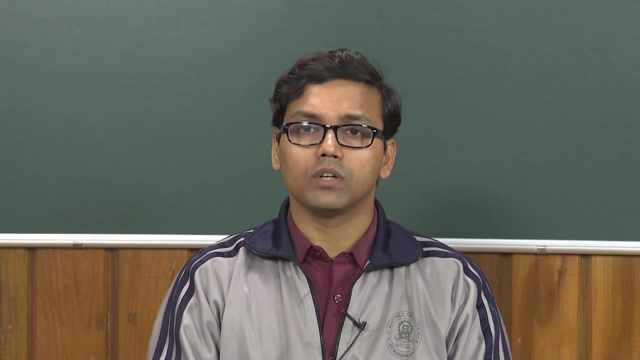 where we use this particular breeding reaction to produce uranium 233.. And Subsequently, that uranium 233 is used as the primary fuel isotope, And breeding is also plays a very important role in showing the prospect of nuclear energy for future. while the stock of uranium is quite limited, Only through the breeding we can still continue. 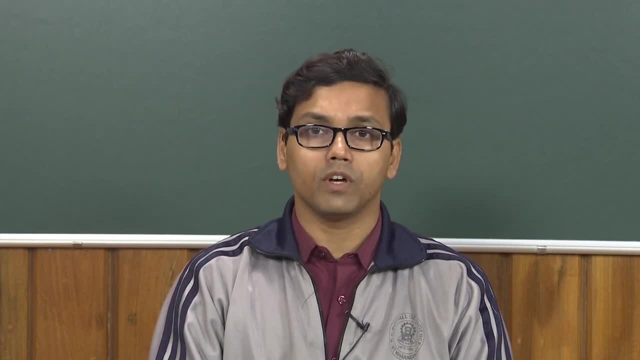 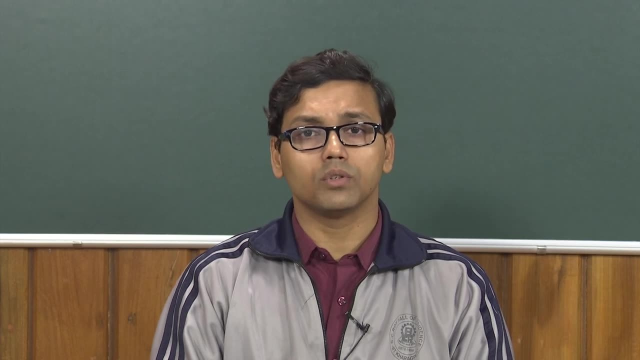 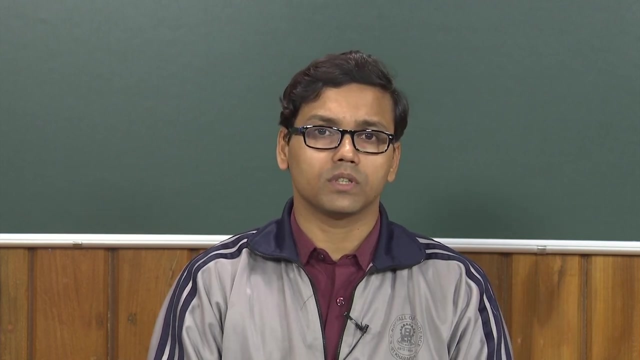 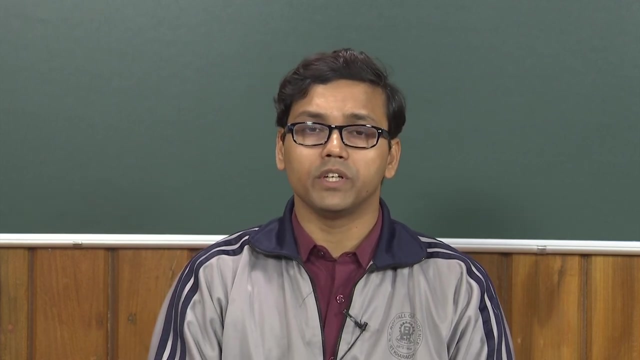 to use nuclear power for something in the range of 25 to 30,000 years, which is near infinite considering the present scale. So as one particular isotope, which is uranium 238, which before up to this module was thought about of no use at all, it can be found to be of great significance through this breeding. 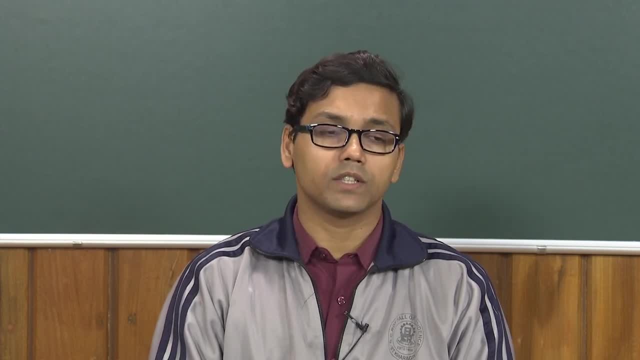 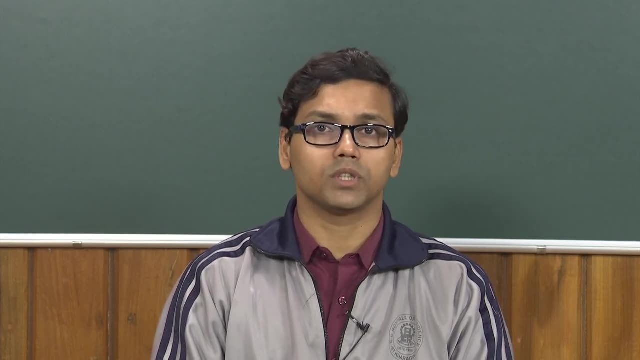 reaction Like earlier. whenever you have discussed about factors like resonance absorption, you must have always felt that that is a loss, Because uranium 238 has a very high resonance absorption cross section at certain energy levels. Therefore, when a neutron of that energy level comes in contact, With an uranium 238 nucleus that immediately gets absorbed, which we have called resonance absorption, and immediately that neutron goes out of the system because that is no longer available to become thermalized and cause any kind of thermal fission, But that neutron which has been absorbed by thorium to uranium 238, that actually can lead to this breeding. 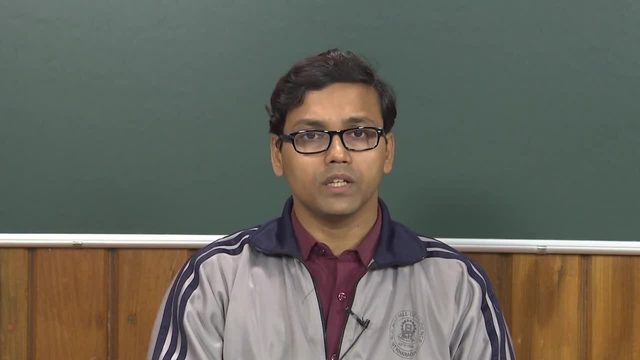 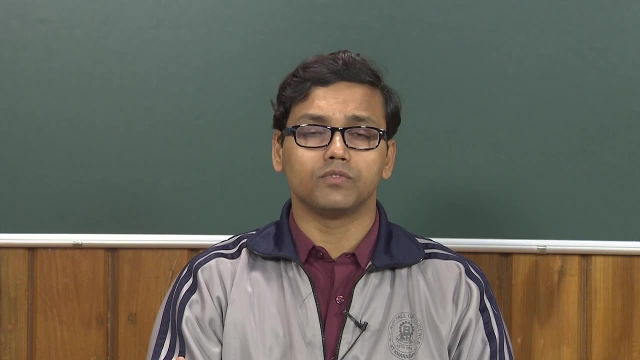 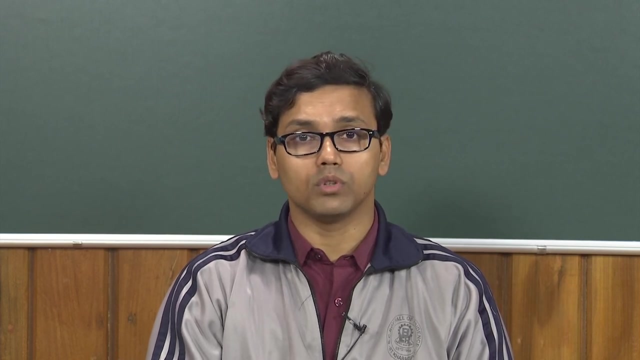 reaction, thereby adding some more fuel into the system, And hence that is also of great importance. And as a result, a reactor, a thermal reactor, which is filled only by uranium can still have 30 to 40 percent contribution in the total power production coming from the plutonium, And plutonium is entirely generated inside. 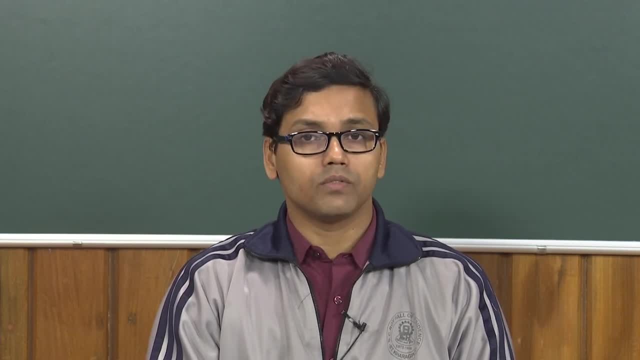 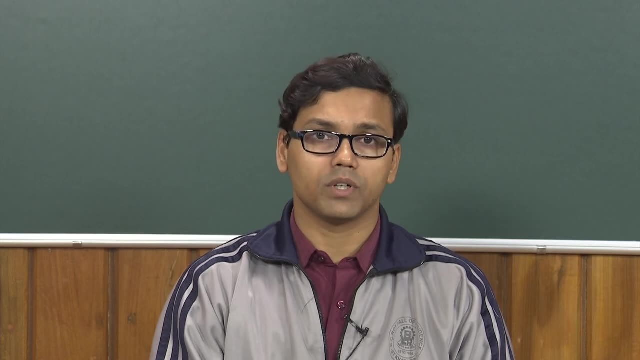 the reactor alone. Breeding ratio we have defined as the ratio of the number of fissile nucleus present after a reaction, divided by number of fissile number of fissile nucleus consumed during a particular reaction. And when a reactor is having a breeding ratio greater than one, then only we call it a breeder. . . . . . . . . . . . . . . . . . . . . . . . . . . . . . . . . . . . . . . . . . . . . . . . . . . . . . . . . . . . . . . . . . . . . . . 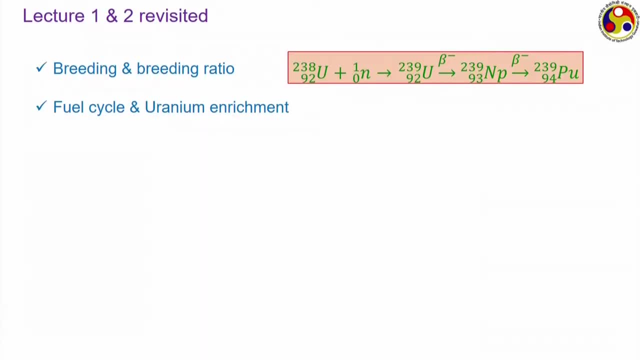 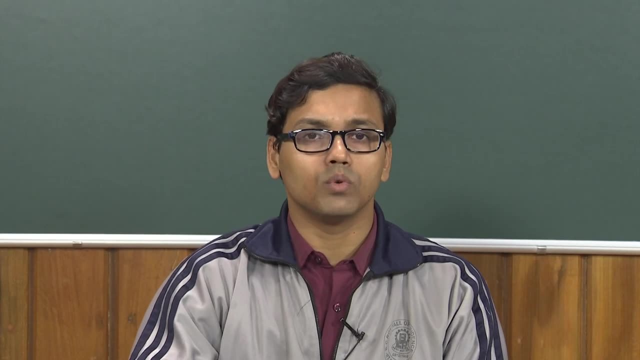 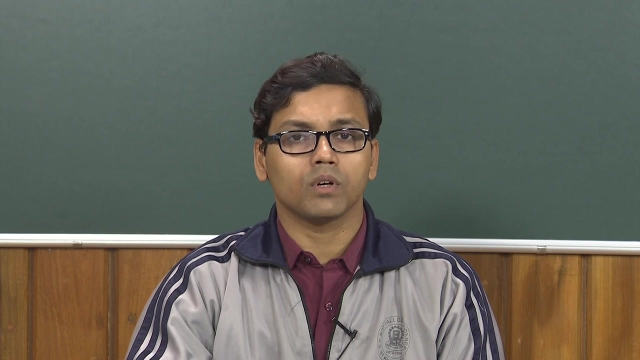 ah, We have discussed about fuel cycle and the neutron or uranium enrichment process in the previous lecture. While we get only raw uranium ore from the mines, that needs to go through the milling and conversion processes. Out at the end of the conversion processes we get uranium hexafluoride gas which goes through this enrichment process. there are 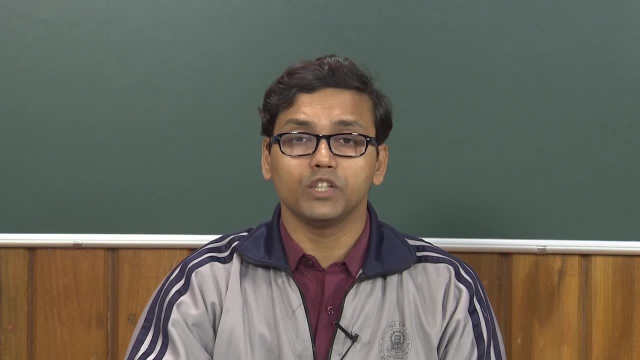 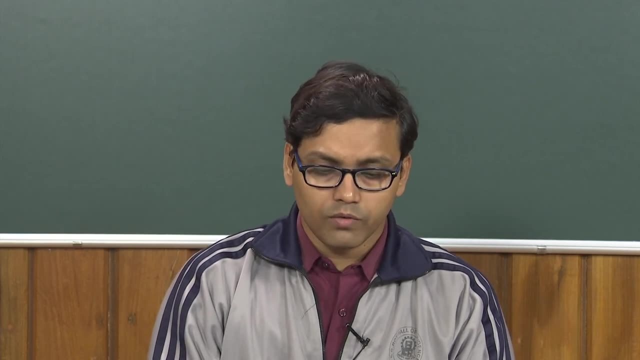 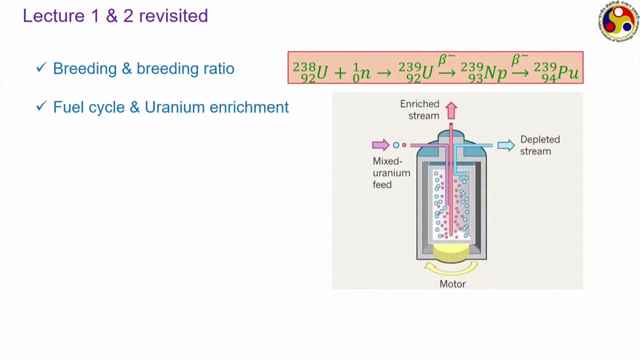 several ways we can achieve enrichment. Basically, enrichment refers to a process which increases the fraction of uranium 235 in the total mixture, And out of all the possible methods, this particular one, which is the gas centrifuge, is the most popular one at the present, but the laser 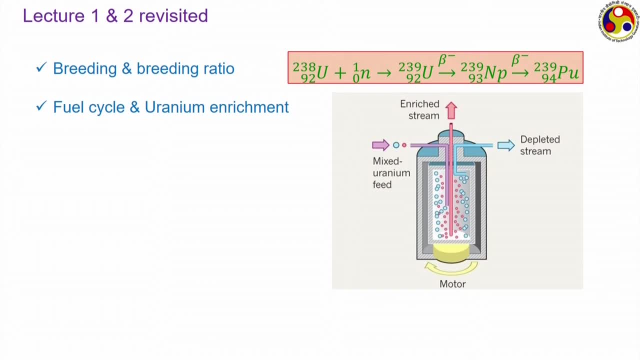 one. also. the laser based method also has a great future ahead, probably So. once we get a stream of uranium which is enriched, that is, which has higher fraction of uranium 235, that is subsequently taken to the nuclear plants, The nuclear reactors, for utilization, and also, once the entire process is done, the spent. 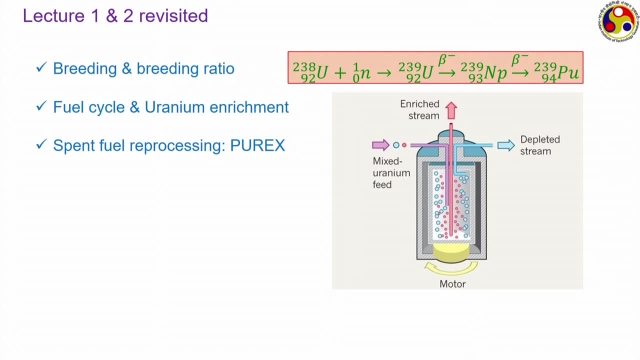 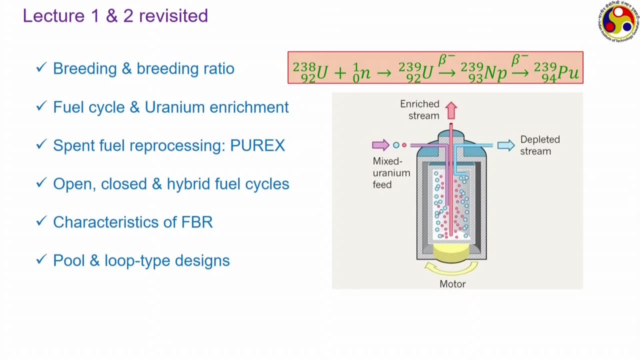 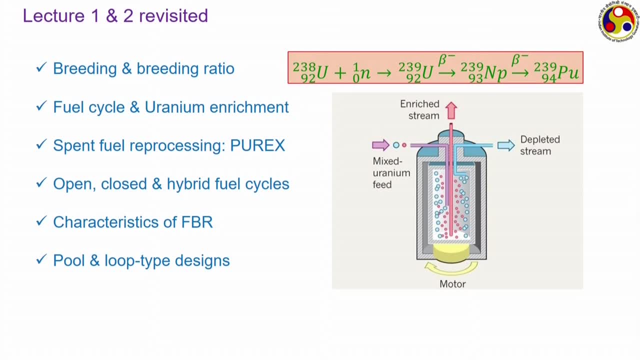 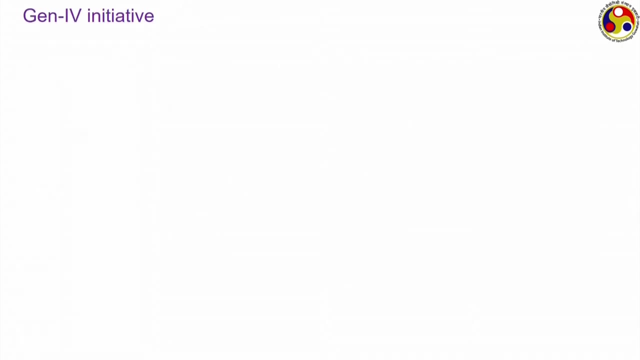 reactors and then to facilitate that which will mostly we discussing about the coolants that we normally use in breeder reactors. But one question I should answer at this point, that why we are talking about breeder reactors in such depth, like in the previous module. 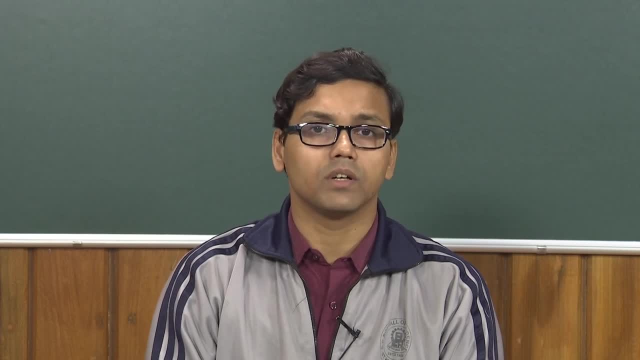 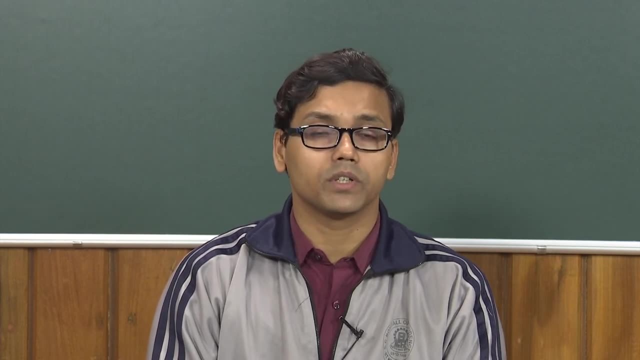 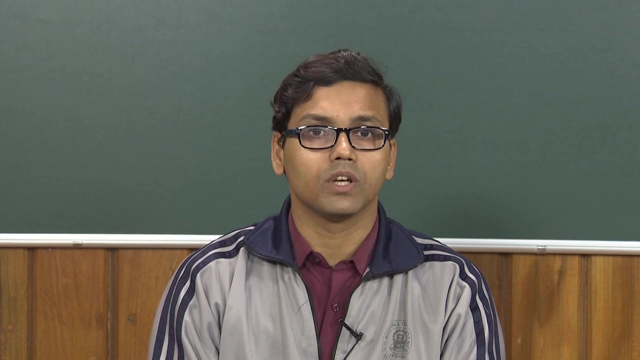 you talked about thermal reactors And there are a several types of thermal reactors have a level, like the pressurized water reactor, boiling water reactor, pressurized heavy water reactor, gas cooled reactor or the RBMK group, which is graphite moderated light water reactors. So there are so many variations, but still we went through them. 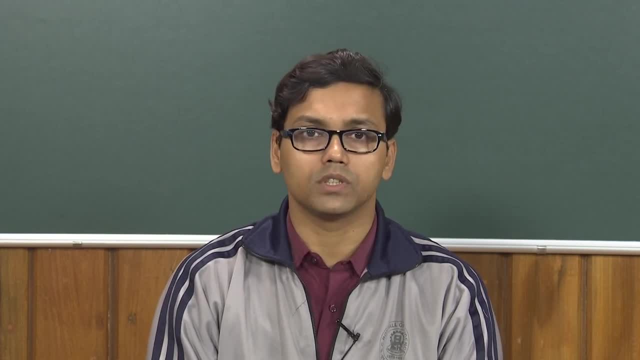 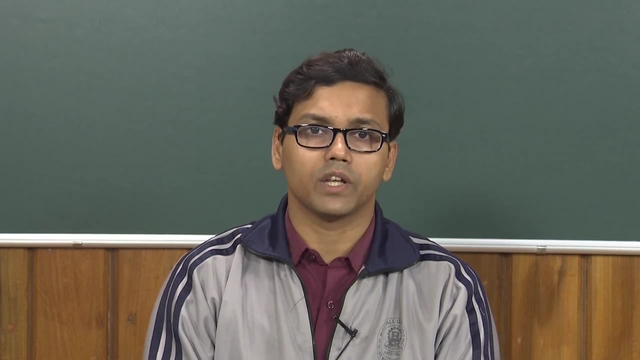 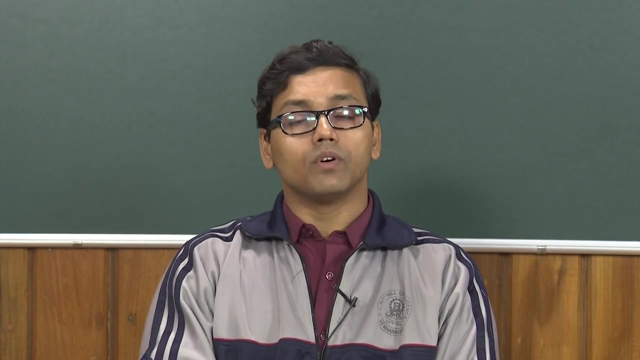 quite quickly and quite quickly and finish that module in just two lectures. But in this FBR group we are discussing in more detail and taking our time to discuss. that is because of this generation 4 initiative. Under generation 4 initiative, which basically proposes the future nuclear reactor designs which are going to rule the power production. 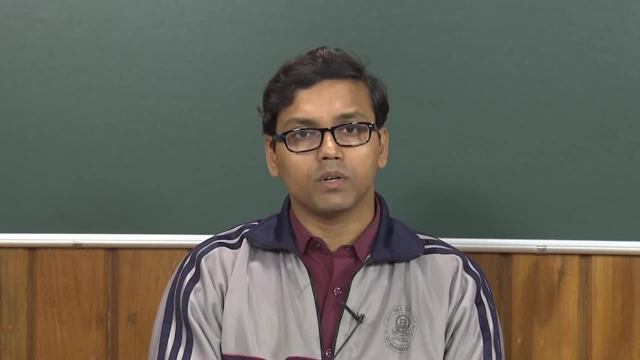 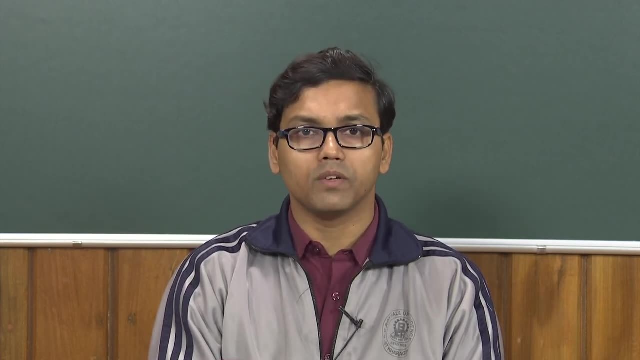 industry in the years to come. If you remember from our previous module, there are generally six reactor designs which are found to be very prospective under this generation 4 initiative. The one of them is this VTR or VHTR, very high temperature reactor. 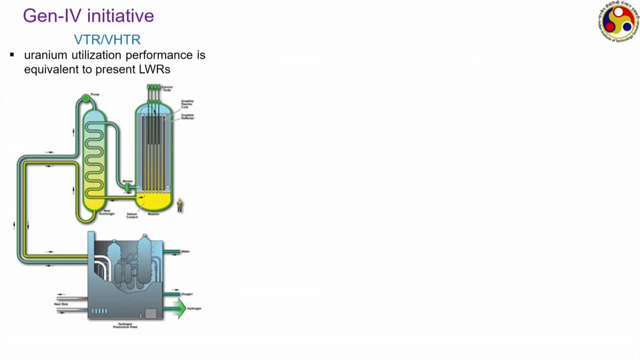 We have discussed this characteristics earlier, but of course, none of the generation 4 reactors are active at the moment. Some, while some of them, are restricted to the research laboratories. some of them are only concept and has gone through theoretical analysis, or very small. 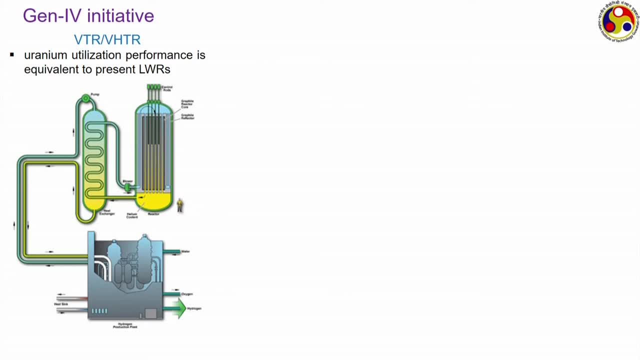 scale test runs Now from the knowledge base that we have gained from there. the VH VTR shows that it has a very poor fuel utilization performance. In fact, its utilization performance is very low. So it is very low in terms of the fuel utilization performance. So it is. 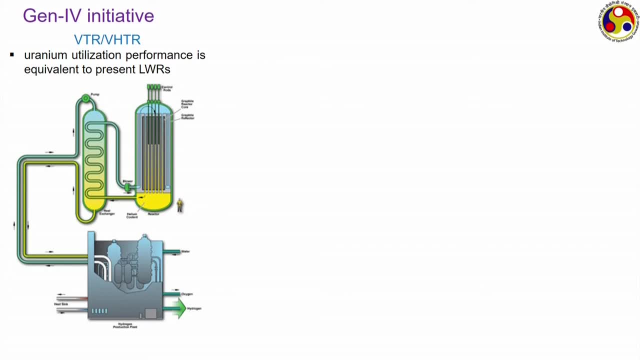 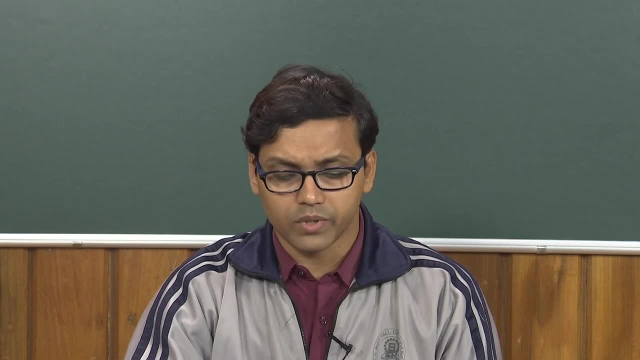 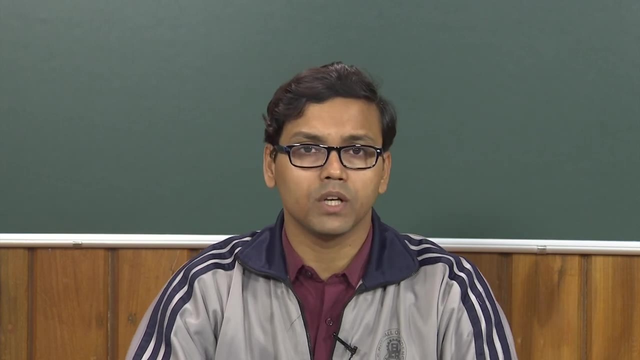 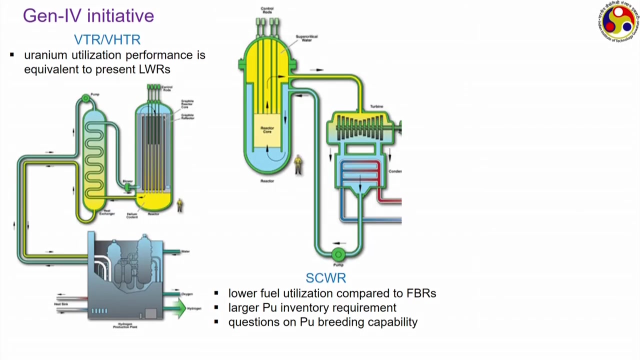 at tastes that VTR weakens his thermal efficiency. However, relation of product is expected to great with this 8 year old VTR at the current rate. other one is SCWR and of course it is very promising because it works at the super critical pressure and temperature. level, And so the PMC works by very high thermal efficiency. Therefore, MZ energy is commercial. meaning this: Aomal g P Republicans, the at the unit that the man is releasing ahead used gensان g emersion Japan, and that is only fashionable battery. It is a proper ingredient. 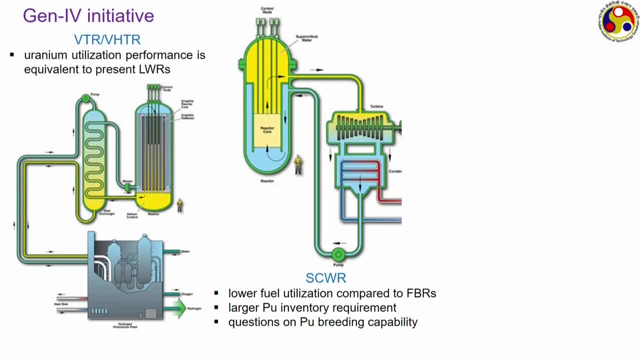 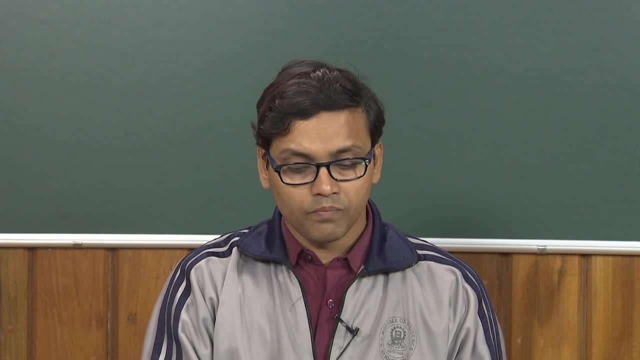 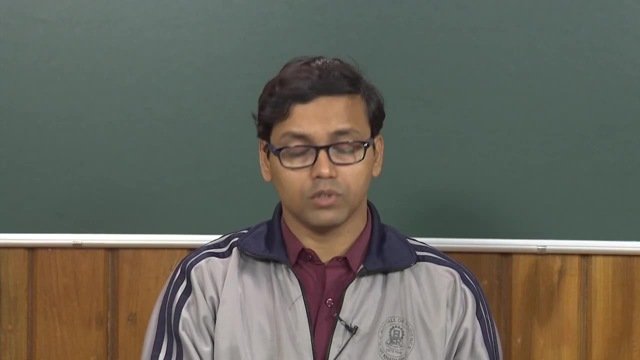 range of 44 to 45 percent, but it has own issues like very high pressure and temperature and also from fuel utilization. performance point of view its utilization is lower compared to the present FBRs. The present design fast reactor shows a much better utilization of the fuel, and better fuel utilization means much less amount of waste product, So lesser effort is required for the waste disposal. ACWR fails in that category And as the fuel utilization is poor, so it requires much larger fuel inventory, particularly a plutonium inventory requirement, And also it has some questions raised about the plutonium. 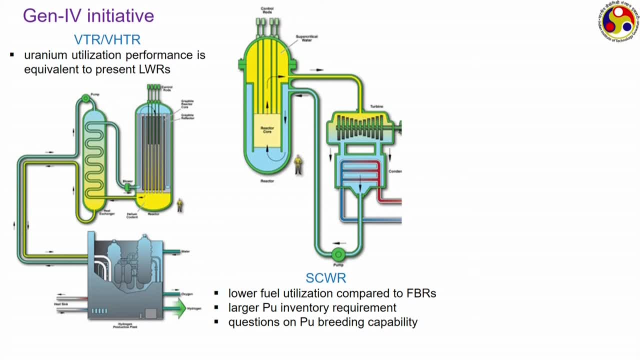 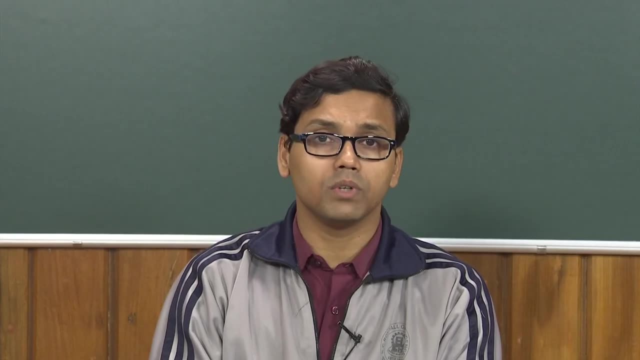 breeding capability, which still it still needs to, or it is still not in a position to demonstrate a very high breeding ratio, And therefore doubt remains whether we at all can go for this ACWR in future, Because whatever future reactors we are going to have, 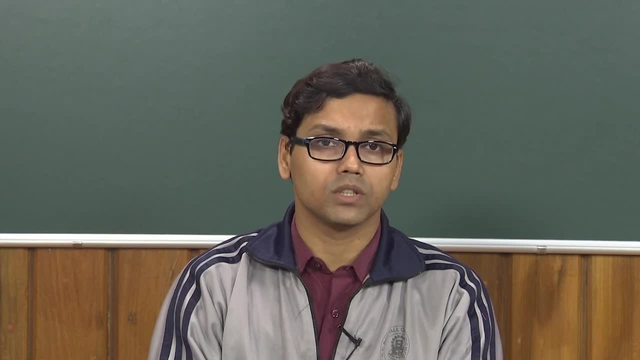 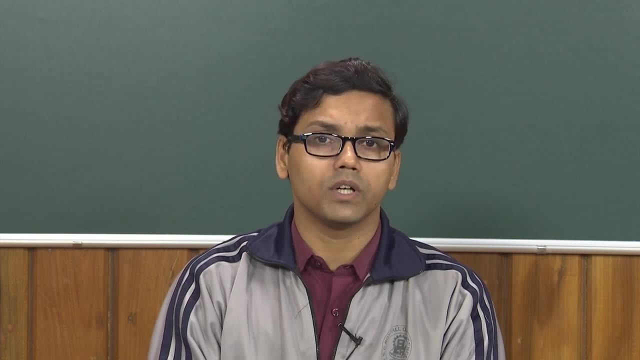 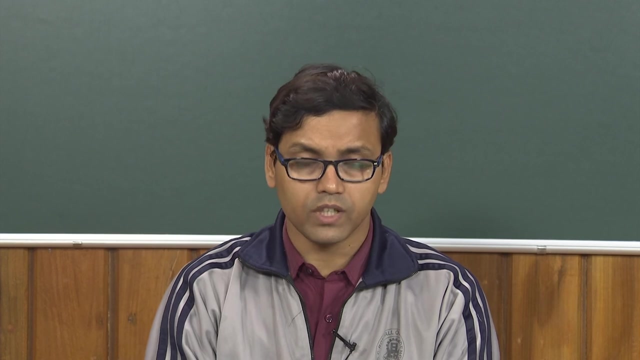 Under this generation 4 or maybe even future generations. we must ensure that breeding, a proper breeding ratio or high breeding ratio, is a must So that we can get a good fuel economy, a very high utilization of the fuel. but both VHTR and ACWR fails in that category. 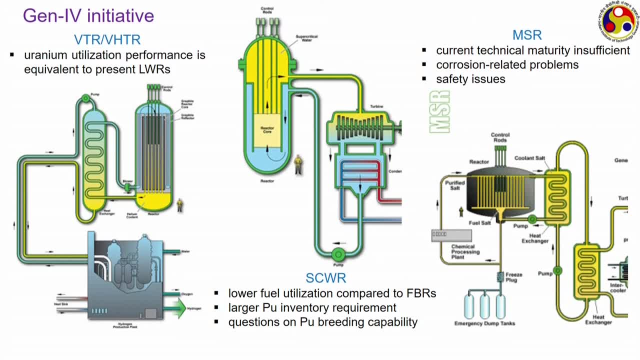 And the other one is a molten salt reactor. Here the knowledge base is quite small. In fact the technology itself is not very matured, And still lots and lots of R and D is required on MSR before it can at all be realized It. 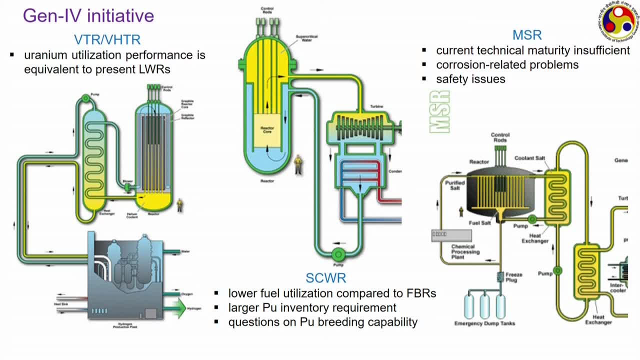 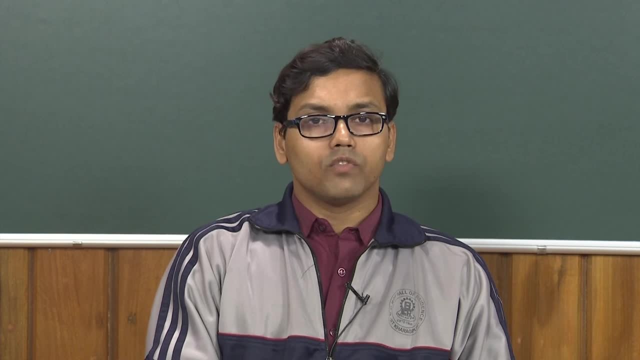 is still a concept which has hardly got tested at the laboratories And as the molten salts are used here, So there will be a big amount of corrosion problems And the safety issues, or maintenance issues, are also very much prevalent for MSRs. Therefore, out of the 6 designs, 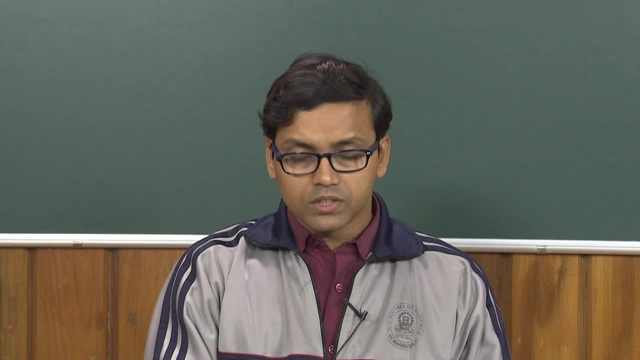 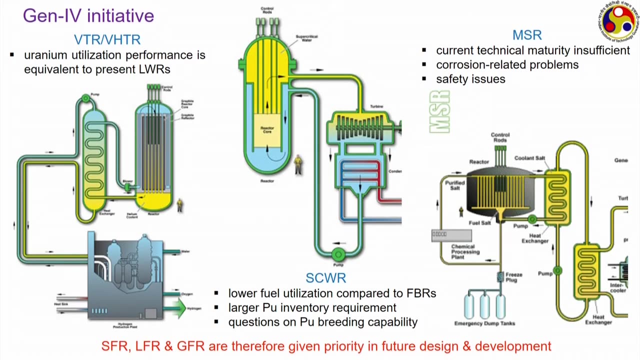 selected in generation 4.. or this 3 have their own issues, which leaves us with the remaining 3, that is, SFR, LFR and GFR, or namely the sodium cooled fast breeder reactors, lead cooled fast breeder reactors and gas cooled fast breeder reactors, which have given priority in future design and development. 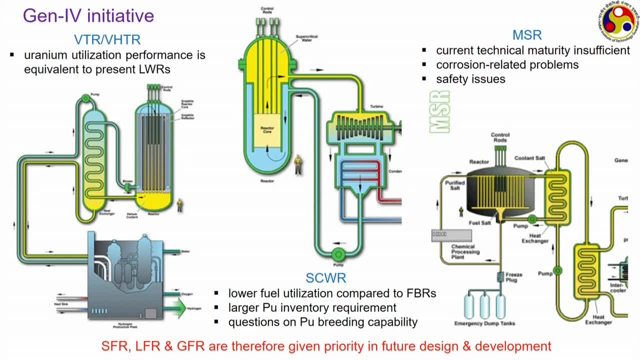 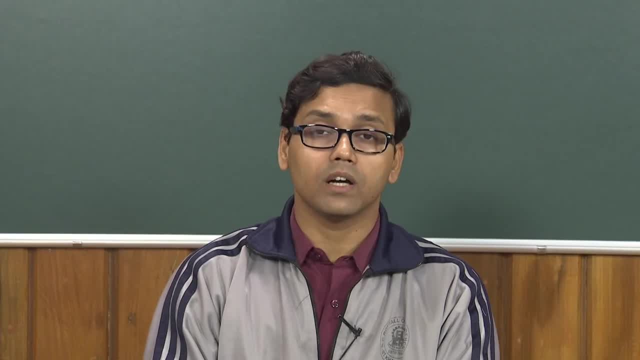 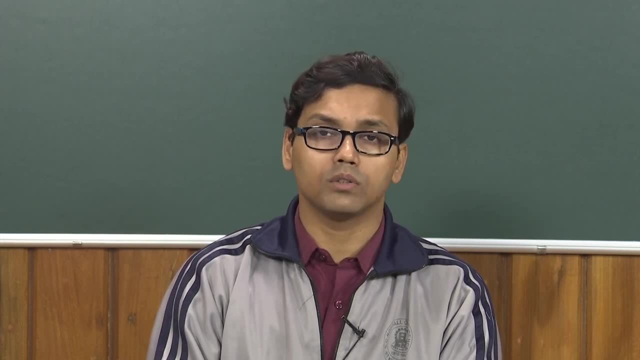 and, incidentally, all of them are fast reactors. and that is the reason we are discussing so much in fast reactors or a fast breeder reactors, because fast breeder reactors are the future, The present day that is under generation, to all those PWRs and BWRs or all those thermal 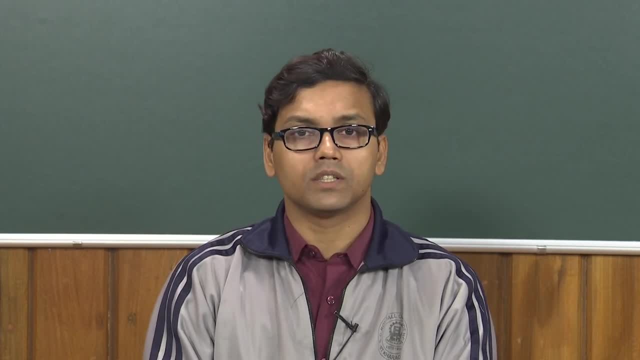 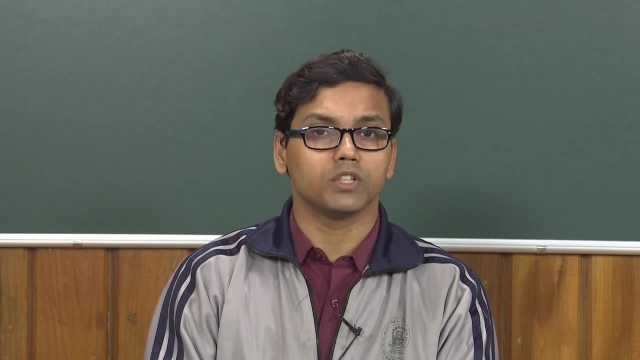 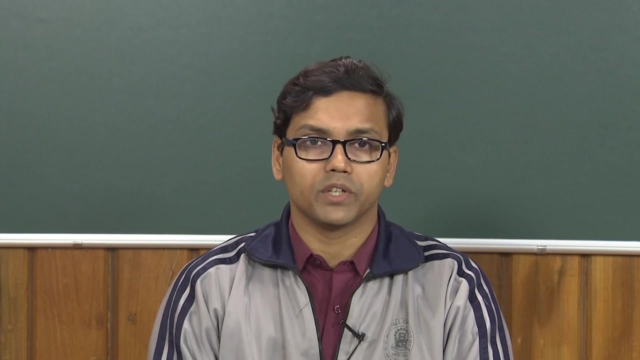 reactors that we are using at the moment. in next 3 or 4 decades to come, they all may get extinct and slowly but surely they will all get replaced by the breeder reactors, and that is why it is very important to get some more idea about the breeder reactors. 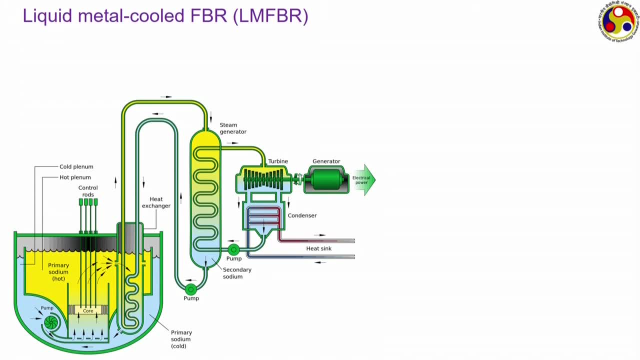 Now most common design of breeder reactor is this LMFVR, or liquid metal cooled FVR. and this particular picture we are seeing from the beginning only where we are using a liquid metal, generally liquid sodium, as the coolant. This design, can you guess it is a pull type or loop type. sure it is a pull type design. 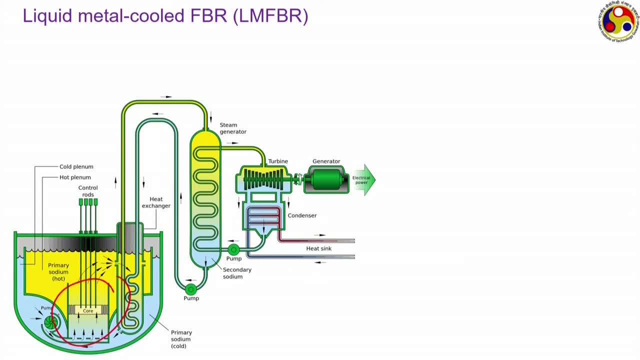 because here you can clearly see the reactor core, the primary pump and also this intermediate heat exchanger. all of them are immersed into this big pool of sodium, big pool of liquid sodium. So as they are all immersed into this big pool of liquid sodium, we call it a pull type. 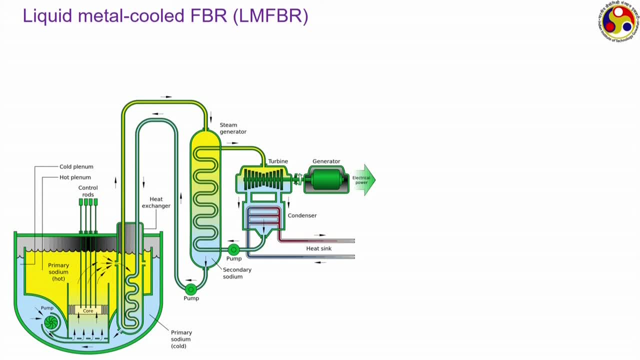 design. The cold sodium or cold liquid sodium is allowed to be pumped through this line into the core, where they gets the energy. So it becomes high temperature sodium, which is termed as a primary sodium here. This high temperature liquid sodium passes through this intermediate heat exchanger through. 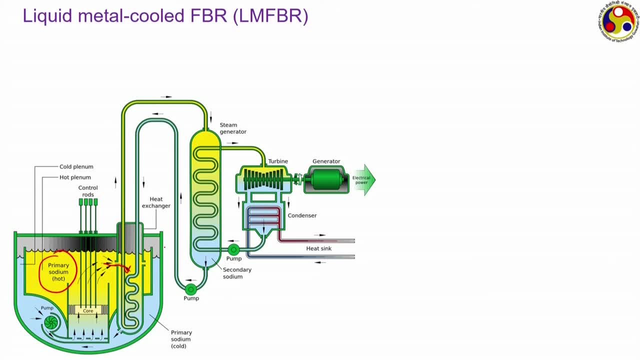 this line and there it passes this energy to a secondary heat exchanger where the working medium is also liquid sodium. So the liquid and then this primary sodium comes out from here and then again gets pumped through back to the core. But the liquid sodium which is flowing through the secondary circuit that comes via this. 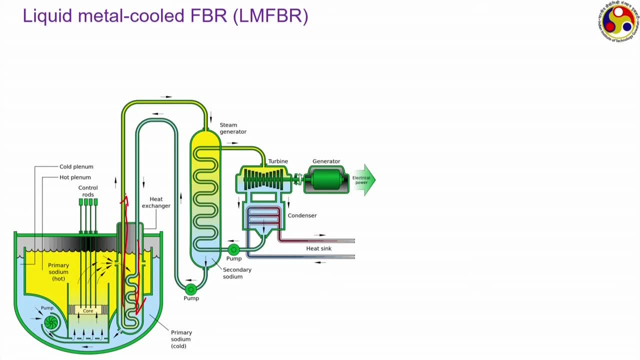 line and then gets the energy And then goes back side and then it goes to the other heat exchanger which is basically a steam generator. Here, on the high temperature side, we have this secondary sodium which has just come out of the intermediate heat exchanger with large amount of energy, and on the primary 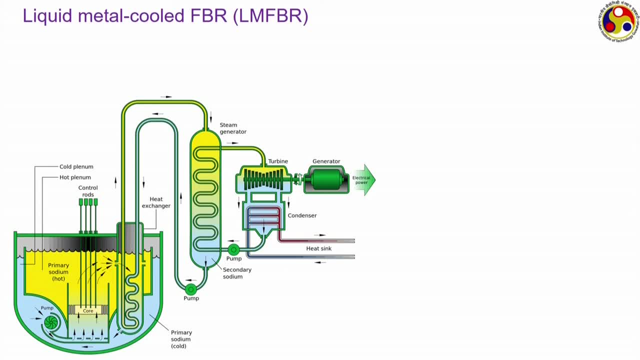 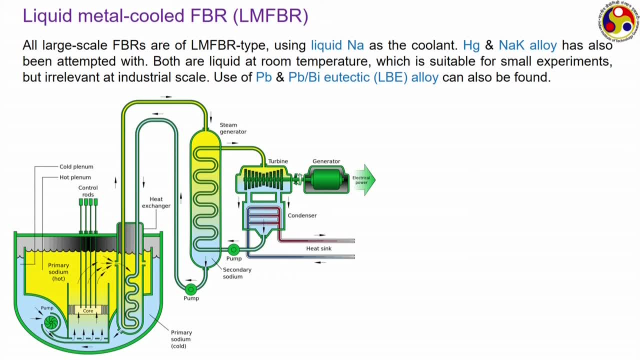 ability, your требability, working medium in the final turbine generated circuit. That is the reason of having this intermediate heat exchanger. 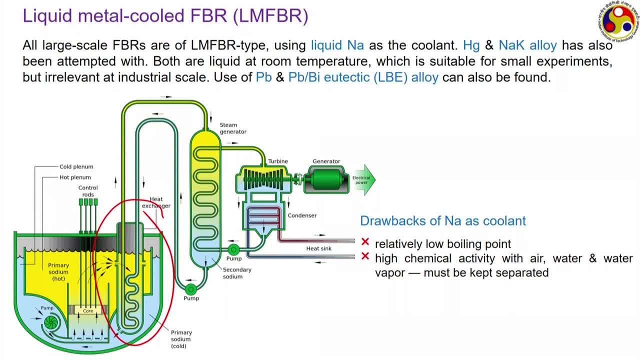 The sodium that we are heating up in the primary vessel and that that we are in the pool, that sodium constant and supply your exchange energy with the steam in the steam, you know. Rather, we are using the secondary sodium load, which is operating at a lower temperature level and also that provides some kind of safeguard So that the sodium 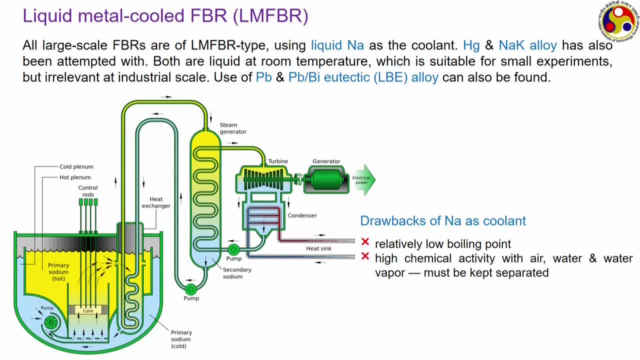 is never coming in contact sodium- in the primary side at least, that is never coming in contact with the water or water vapor. The mean free path of neutron inside sodium is much larger, which increases the possibility of leakage as well. And finally, another problem which happens generally in the energy interval of 0.7 to. 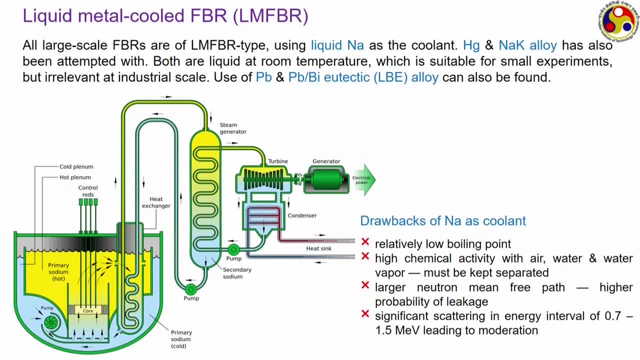 1.5 MeV. the scattering cross section of sodium with within this particular energy level is quite high, both elastic scattering and inelastic scattering, And therefore there is possibility of some kind of moderation effect that may come in when the neutron falls in this particular. 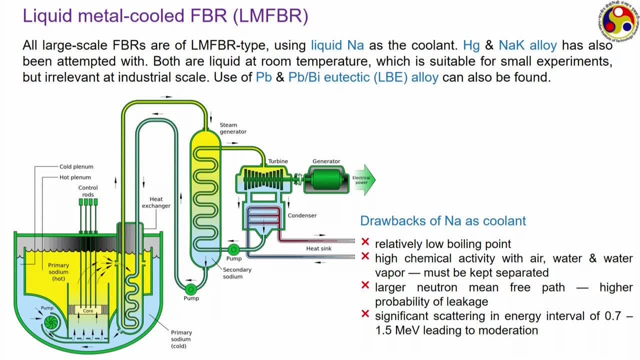 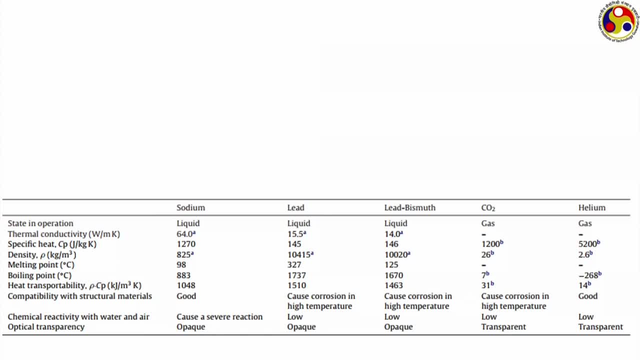 energy band. So these are quite a few drawbacks that we should be careful of while using sodium as a coolant. But sodium has its own advantage also for that. just take a look at this table. Here we are comparing the coolants which are commonly used in generation 4 fast breeder reactors. 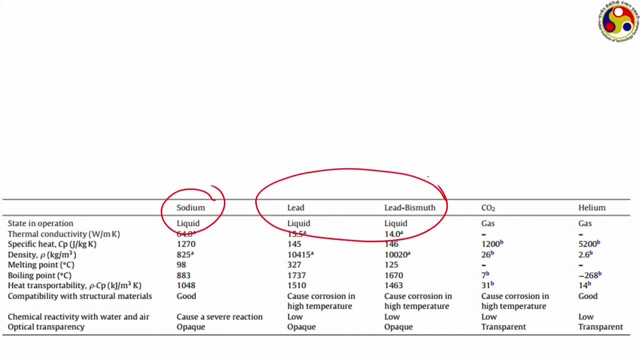 Sodium is the coolant for SFR. lead or lead bismuth, eutectic, are generally thought about for the LFR, and in gas cooled reactors we may use carbon dioxide or, more preferably, helium. Look at their properties, And so the classic cooling reactor is called the LFR, which is a cold reactor, that is SFR. 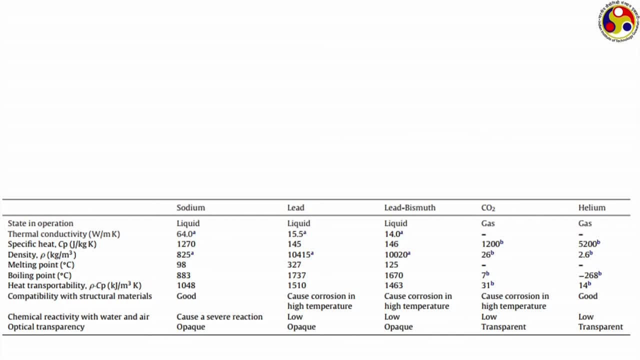 and LFR comes under the liquid metal cooled FBR category, whereas CO2 and helium are used in gas cooled reactors. Now first let us take a look at the melting and boiling point data. Sodium has a melting point of 98 degree Celsius and a relatively low boiling point of just around 883 degree. 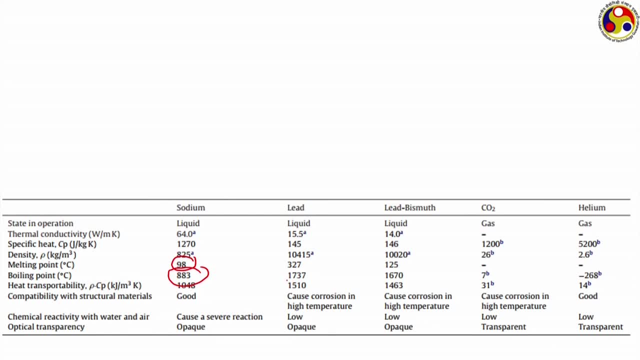 Celsius. Compared to that, lead has a boiling point of 1737 and lead bismuth eutectic is also quite similar. So they have extreme, very, very high boiling point and thereby allowing the coolant to reach much higher temperature, Whereas when you are operating with sodium, 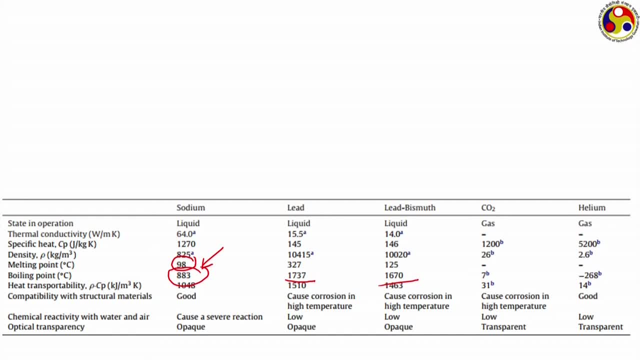 the final coolant temperature may has to be lower than this value. In fact it should be reasonably lower than this. value may be hardly allowing something like 800 or 820 degree Celsius, Whereas with lead or lead bismuth- eutectic- we can go easily up to 1500. 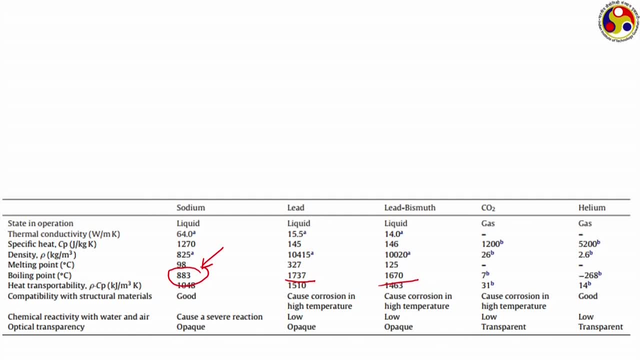 degree Celsius, without ever bothering about the cooling, or rather the phase change of this coolant. The another point that we should consider, which actually is favorable to sodium: Sodium has its own advantages because it has superior thermal hydraulic parameters. Its melting point is not of any consideration, but boiling. 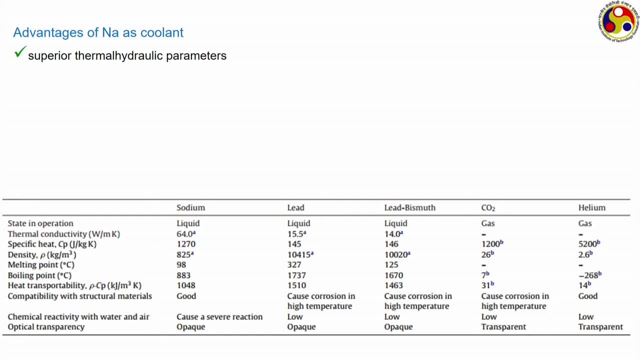 point is. but apart from that, all other thermo physical properties of sodium are excellent, Like look at the thermal conductivity is. thermal conductivity is 64 watt per meter Kelvin, which is just in the order of 15 for lead. Similarly, if you take a look at the 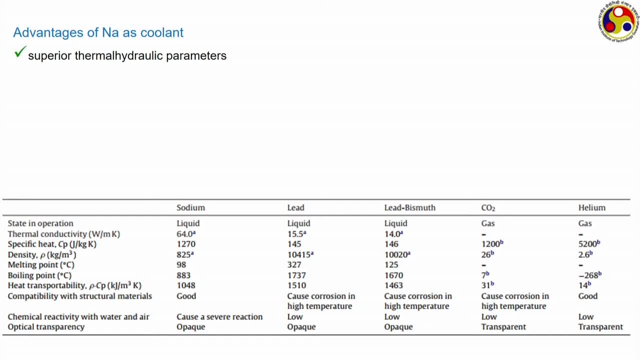 say row CP product, which is also called the heat transportability or heat capacity. It is also quite good for sodium, Of course. lead is even better. both lead bismuth, eutectic and pure lead. they are even better. Specific heat for sodium is much larger to 1270, which is significantly higher than lead. 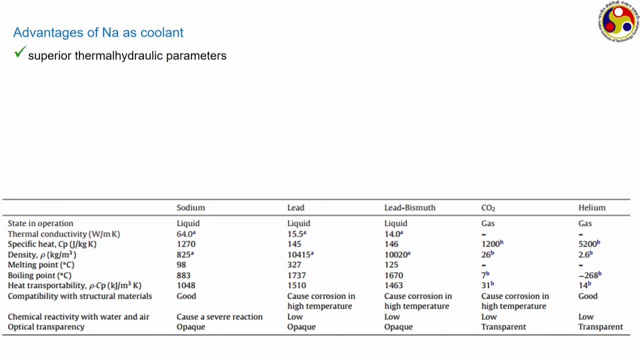 Another big issue that we may have using liquid lead as the as the working medium. sodium is a very, very light metal. So look at the density of sodium: it is around 825 kg per meter cube and this is 10000.. So is this one. So it is about 12 to 14 times larger than lead bismuth. 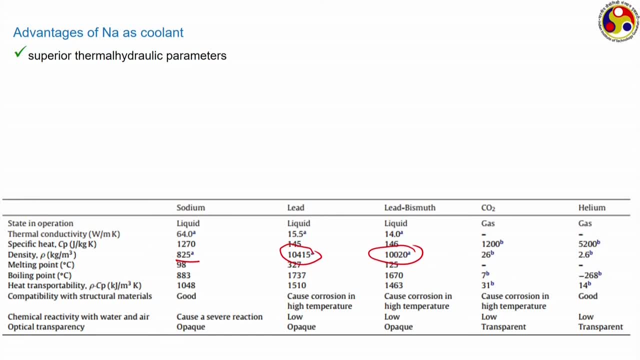 eutectic and 14 times more dense compared to sodium and as it is, as the density is much larger. So signal that in that proportion, the pumping power needs to be introduced, needs to be enhanced. Much larger power will be required to drive this liquid lead or liquid. 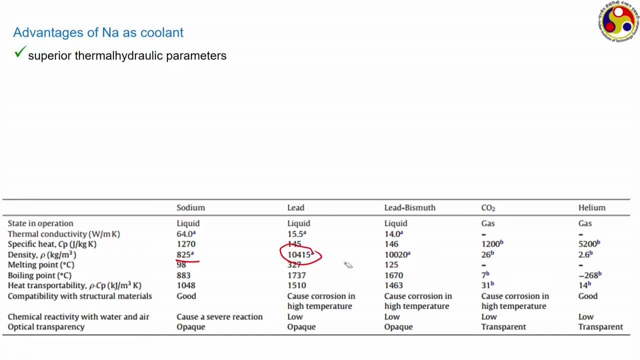 lead bismuth eutectic mixture to flow through this coolant channel or maybe through the around, through the circuits or through the zones around the core, And there will also be chance of pipe clogging because of its high density. So, from all this point considering, sodium has superior thermal hydric parameters and 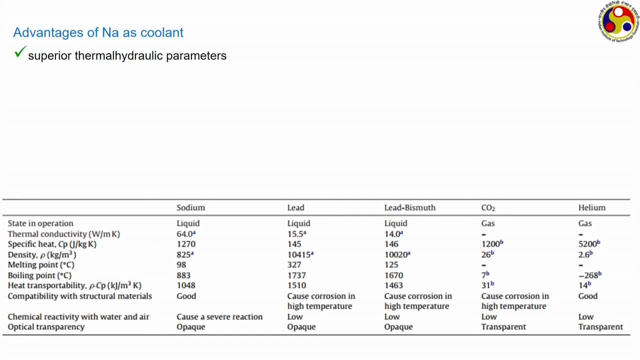 apart from the boiling point, once we can restrict the highest temperature, it is definitely more suitable fluid compared to lead, Melting point is very, very low. lead has a melting point of 370, 27 degree Celsius, 327 degree Celsius compared to just 100 degree Celsius. 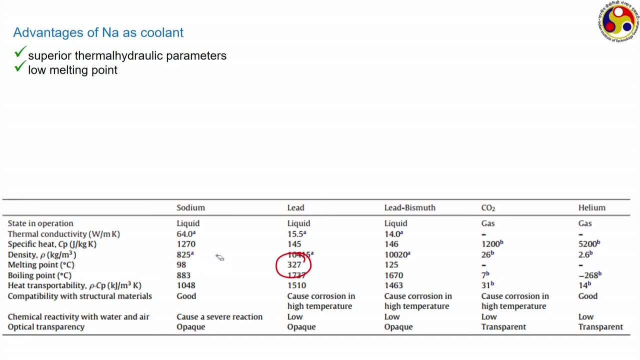 Therefore, while the upper working temperature are allowable, working temperature on the higher side is very high for lead, but the lower side temperature is also quite high. The operating temperature should be something like 350 degree Celsius or higher- the lowest operating temperature- And so we have to generally handle much higher temperature level in LFR and the coolant temperature. 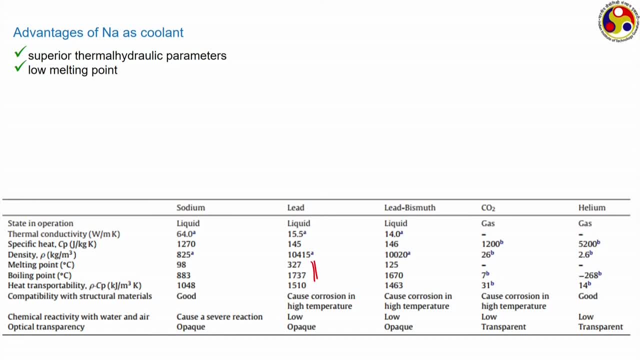 in no case should fall below that 350 degree Celsius. Well, this is an example of a любой. The temperature range applicable for sodium is reasonably wide, like if we compare this range, still we are getting a range of about 700 degree Celsius, but the range definitely. 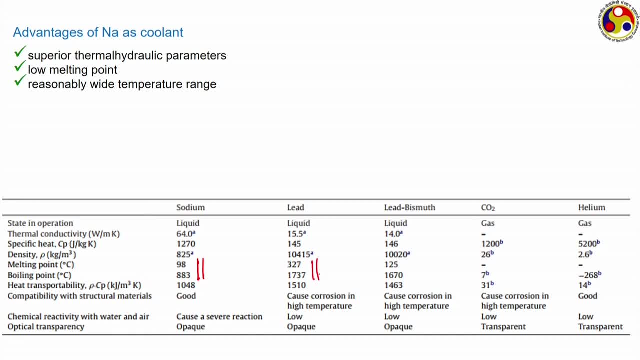 is much larger. in case of lead, where I can find it is around 1400 degree Celsius. So if such kind of high temperature change is desirable, then we cannot go for sodium. we have to go for something like lead or LBE. LBE refers to lead, bismuth eutectic. 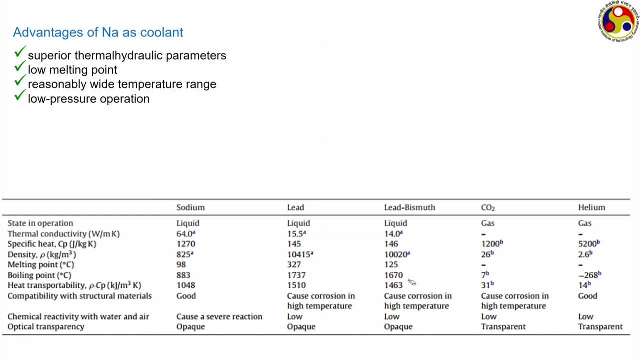 But another advantages for sodium is as the melting point, as long as the boiling point can be managed around that 883 degree Celsius, or I should say as long as the maximum coolant temperature requirement is well below that 883 degree Celsius, We do not need to go for any kind of pressurization. the system can operate under atmospheric pressure. 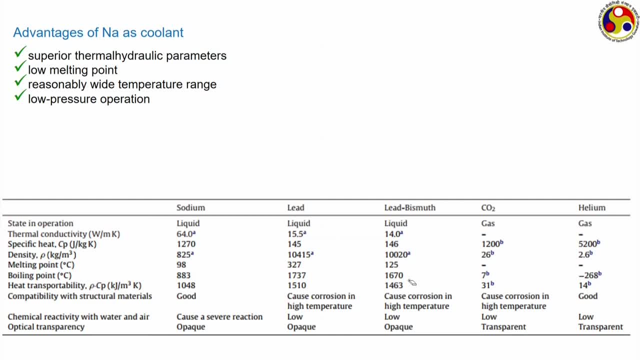 only and still allow a decent temperature range of for operation. Sodium is definitely inexpensive and also it is compatible with stainless steel. therefore, there are several points which generally makes sodium the most suitable coolant, But lead is also not far behind. Lead is. the biggest advantage is compatibility with air and water. 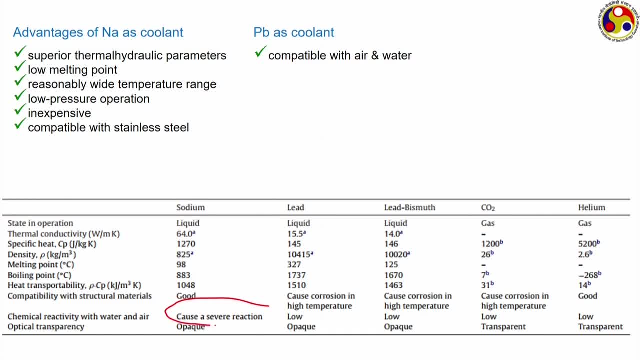 The biggest problem for sodium, as I have mentioned earlier, it is highly reactive, particularly in contact with air and water. it reacts immediately and starts to burn on its own. burn on its own, But lead does not have such level of chemical activity. it is very compatible with both air. 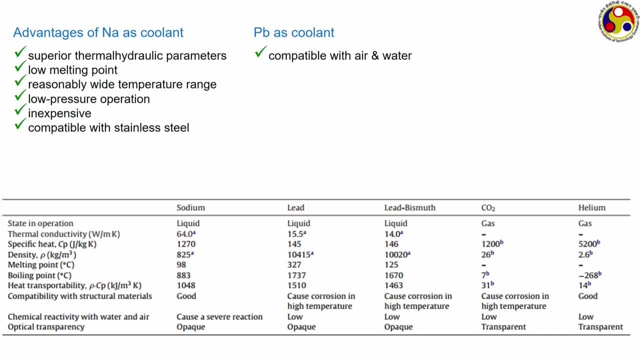 and water, And therefore we can use the lead cooled reactor or LBE. Now let us talk about LFRs, with even open to atmosphere also. or I should not say open to atmosphere, I should say: in case of LFRs, we do not need to have that secondary loop. 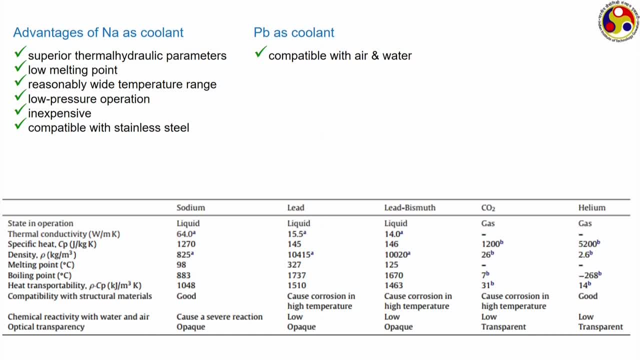 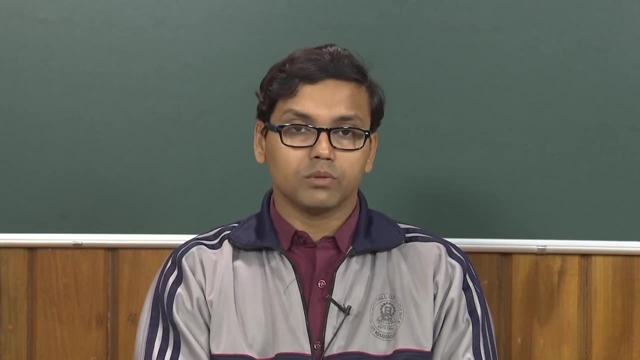 or intermediate heat exchanger loop. In case of SFR, we need that intermediate heat exchanger because the primary coolant, which is liquid sodium, that should not come in contact with the water which is flowing in the external circuit. that is why we use that intermediate circuit where the working medium is again. 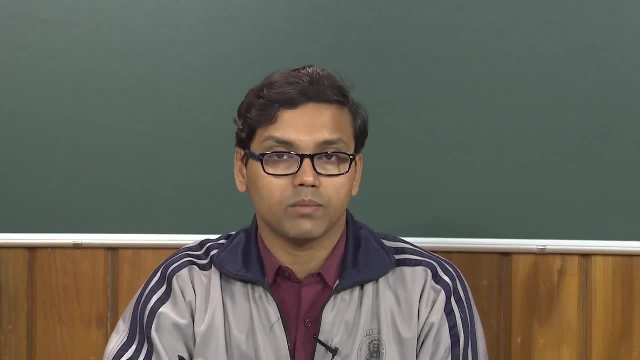 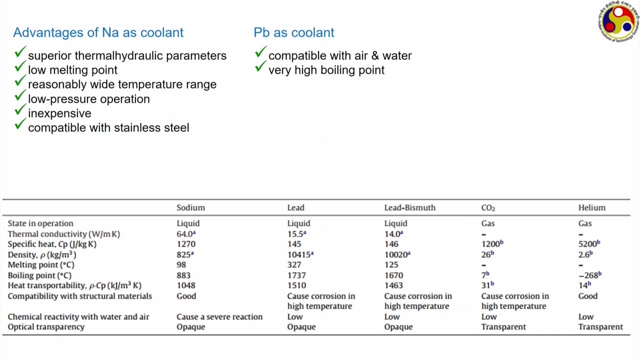 sodium, but working at a much lower temperature level, and that can supply energy coolant. Another advantage for lead is very high boiling point, which I have just mentioned. we can easily go up to 1600- 1700 degree Celsius. heat capacity for lead is larger, like if we compare the: 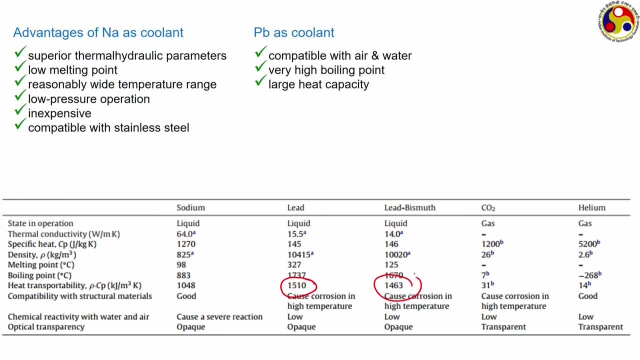 heat capacity? it is 1510. it is 1463 for LBE, So about 50 percent larger than what we get with sodium. And what can be the advantage of having a high heat capacity? I hope you can guess, because we know that for any incompressible liquid we can always write Q equal to m, C, p, delta. 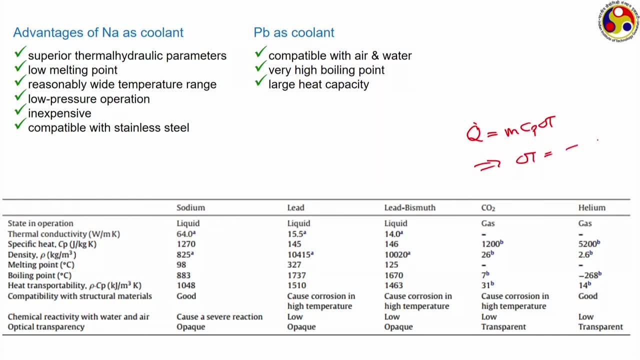 T or delta T is equal to Q by m. sorry, Thank you. And if we break the C p then becomes cross section area, rho C p into cross section area, into the velocity of the liquid coolant and therefore higher the rho C p value, the smaller. 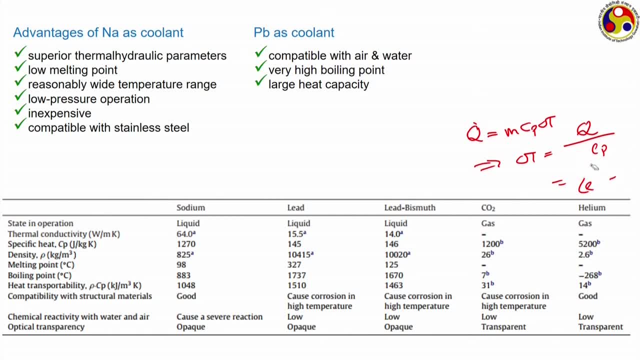 will be the temperature difference of the coolant. But lead or LBE both have quite high heat capacity compared to sodium and therefore they can be more preferable from temperature rise point of view. Sodium lead, like similar to sodium, can also allow low pressure operation. it is also inexpensive. 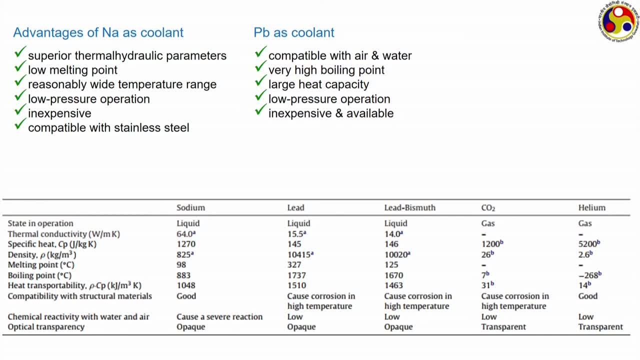 and quite easily available. But lead has its own issues. it is chemically toxic, Which sodium was not. it is chemically toxic and its melting point is very high, like 327 degree Celsius here. So in no case the coolant temperature in the core should fall close to 327. it should. 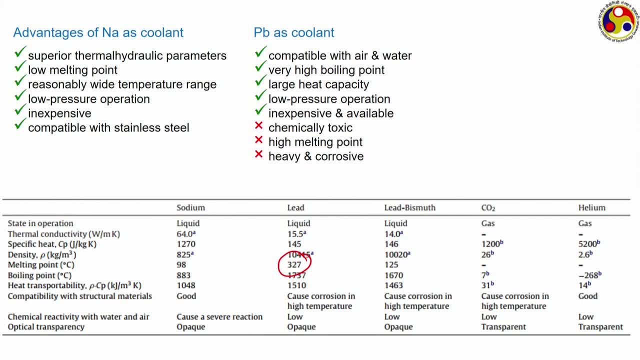 always remain something like 350. Another problem is heavy and corrosive. it is extremely corrosive and so can damage the metals of the walls, And if we look at the heat capacity of the liquid coolant, it is quite high, So we can say that it is very high heat capacity compared to sodium, which sodium was not it. 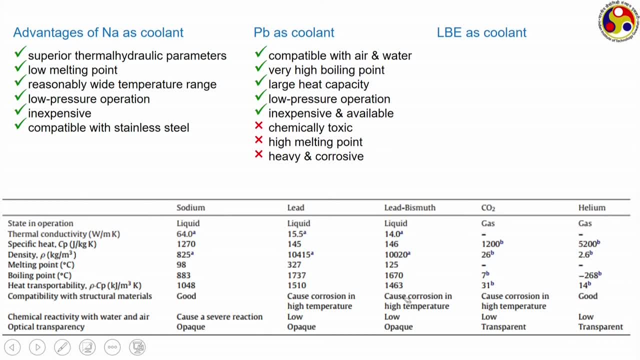 is chemically toxic and its melting point is very high, like 327 degree Celsius here. So in no case the coolant temperature in the core should fall close to 327. it should always remain something like 327 degree Celsius here. And if we talk about LBE, LBE shares most of the issues of lead means from advantage. 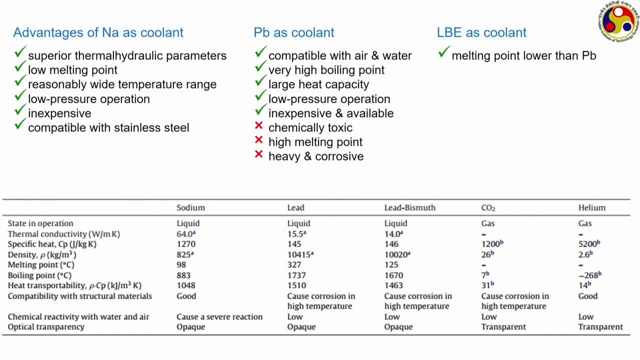 point of view. again, its melting point is: its melting point is lower than lead, but not by a huge degree, and so that is quite decent. Or I should say the melting point of LBE: while it was 327 for lead, it is just 125 for LBE. 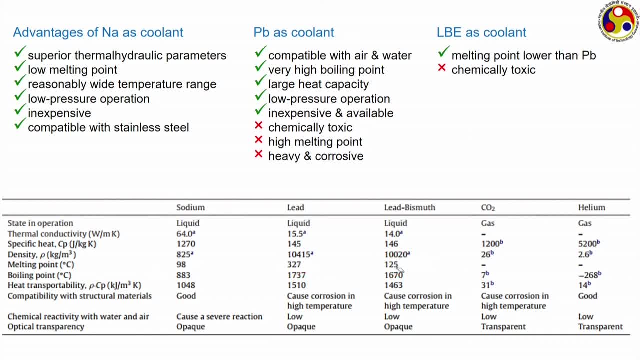 which is quite close to the value for sodium. So we can use LBE and we can allow it the temperature to drop to something very close to the ambient temperature, or ok, let me correct- melting point being so low for LBE we can easily operate at much lower temperature level compared to lead. 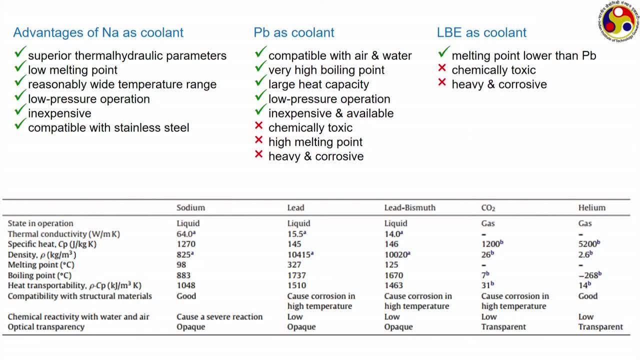 But it has other advantages like similar to lead, this chemically toxic, its heavy and corrosive. then there has been maintaining issues. LBE has not found used in power So far, but there are a couple of a couple of examples where LBE has been used as the 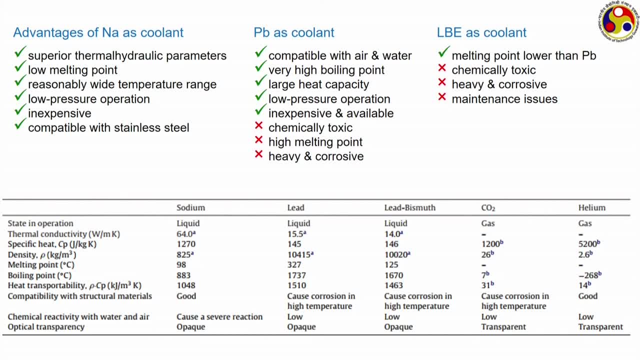 fuel in nuclear power submarines, in Russian submarines, and both cases maintenance issues are found. There may be some other reasons also, but on both to those two Russian submarines, both reported severe maintenance issues and that was related to the flow of this LBE itself, and bismuth is not that easily available. 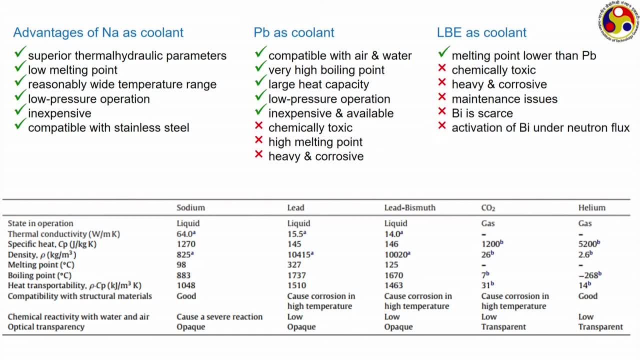 Lead, of course, is easily available, but bismuth is quite scarce and also it can become active under neutron flask Bismuth can participate in a reaction like this. the Bi 2 0- 9, which is the most common isotope, can absorbs a neutron to produce Bi 2: 10 and then it can go through a beta decay. 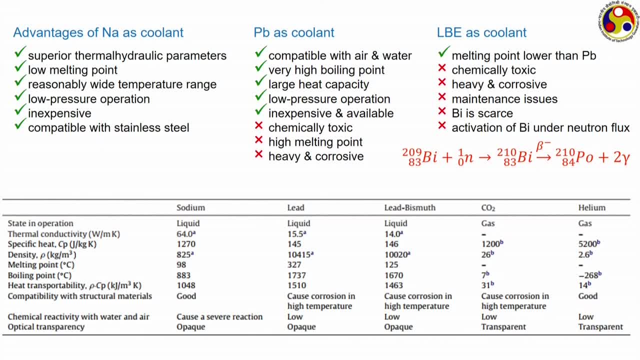 to produce polonium 2, 10, but sodium, if we compare with that, that can also participate in such a reaction, Like sodium 2: 2, sodium 23, which is the most common isotope of sodium which is available in the nature in the form of natural salt, also sodium chloride that can absorb the neutron. 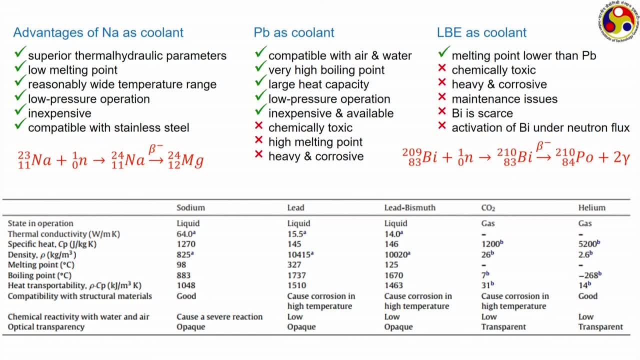 to produce sodium 24, which is highly reactive andimmediately goes through a beta decay process to form magnesium 24.. And you can see the half-life value for Sodium 24. it is half-life is quite smallit is just about 15 hourstherefore from the point. 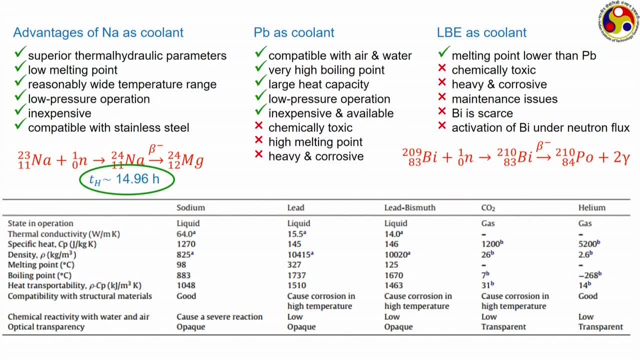 at which the sodium 24 is formed, almost within about 15 minutes, half of those new nucleus or new nuclei willbreak down or will participate in the beta decay to form magnesium and it is expected that this, or we can visualize this conversion, Or we can visualize this conversion of sodium 23 to magnesium 23, to be almost direct, because 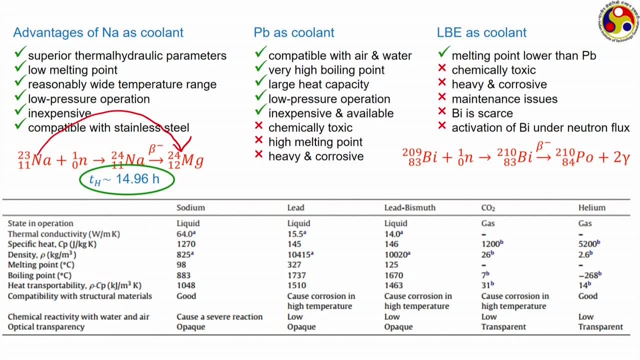 of this small half-life, and magnesium 24 is a stable isotope, So the radioactive effect of sodium 23 inside the reactor is not that significant. but if we compare that with bismuth 2: 0- 9, then half-life of bismuth 2: 10 is more than 5 days, so some 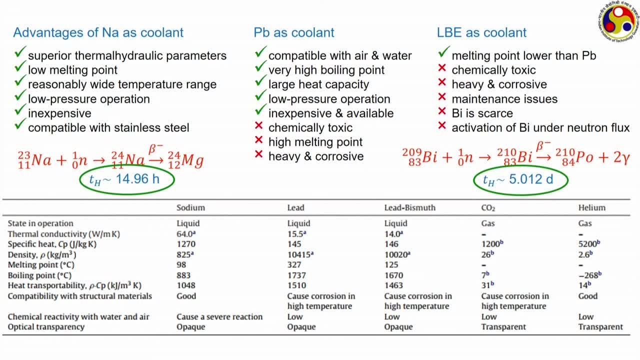 more time is required to remove the radioactive waste From the reactor, no end. also the radioactive waste orproducts like polenum, colour etcetera, which remains inside the reactor. that, or I should not polonium, I should say thisbei 210 now has more time insidethereactor to participate in the radioactive decay. thereby 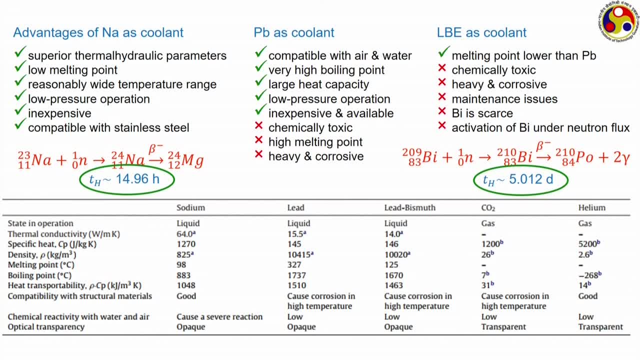 emitting or thereby causing the probability of more radioactive waste. However, making more space, this wasting, the own of radium, is not gloating And the radioactive temperature is very high. The brind here is very low, with cavity and the presence of PM 2 really absent in the 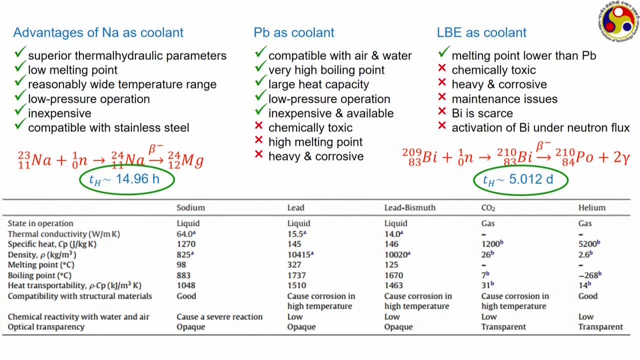 reactor. So, in a nutshell, whatever we are getting from this slide, in the previous slide, sodium has its own issues, but still it is the most suitable coolant that we can identify at the moment and that is why. ah, So the liquid cooled first, beater reactors, whatever we have at the world and the commercial. 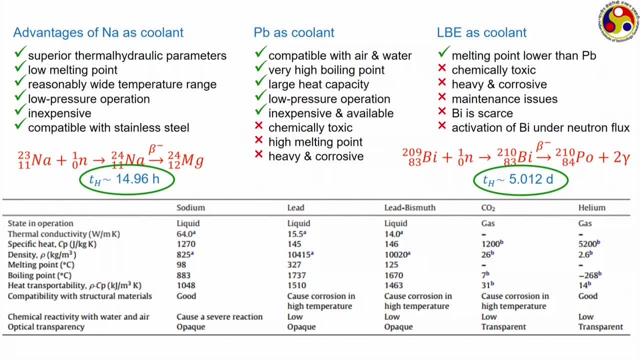 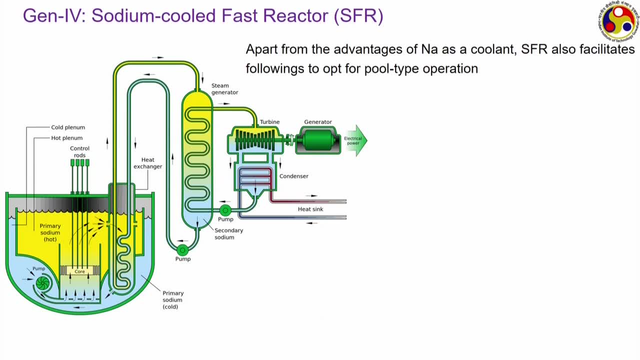 level at the moment. they all work with liquid sodium. So we come to the sodium cooled first reactor, SFR. its characteristics were discussed as a part of the previous module. now we discuss about some issues that it may have. thus sodium has its own advantage, as we have mentioned, but SFR also facilitates for couple ofadvantages. 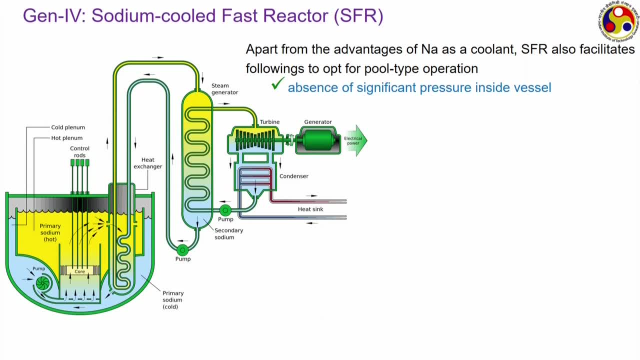 because of which it goes for the full type operation. Pressure is pressure inside the pressure vessel is can be quite low. sodiumhas a low melting point and reasonably high boiling point and therefore we can operate this in unpressurized situation. So this is what we have discussed in the previous module. now we discuss about some. 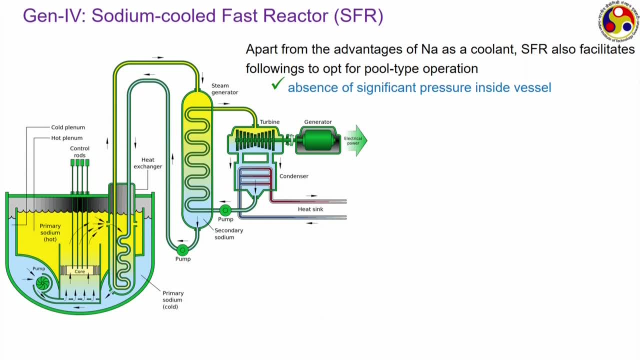 issues that it may have And pressure vessel can remain at the atmospheric condition. Another problem that- or another advantage rather, SFR processes- is a minimal risk of leakage of the primary sodium because the way it has been designed the primary coolant will not leak out the core. but there are several issues which also need to be sorted. 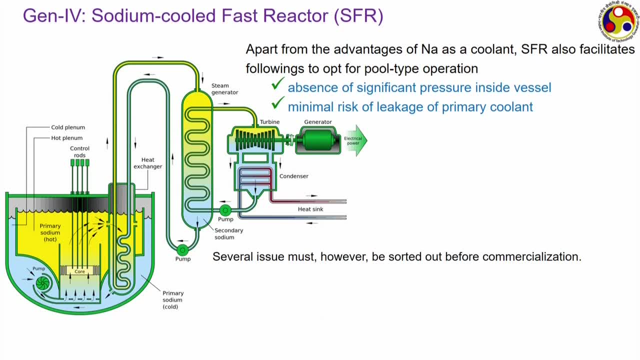 out before full commercialization. Actually, out of this, three SFR, MFR and GFR. 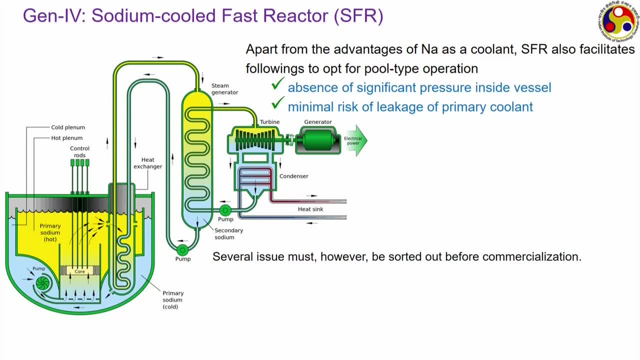 S F? R is the one whose development is at the most advanced stage. the trial runs all. 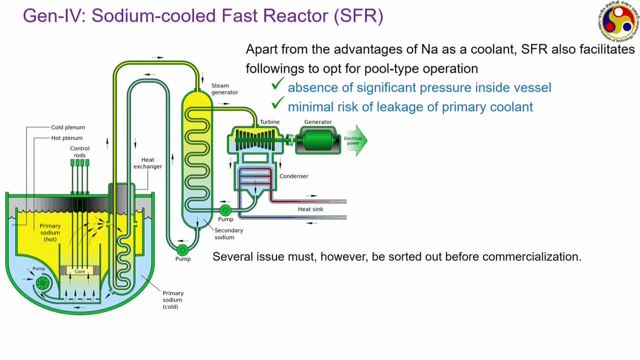 are completed and it is presently gone for the power testing. and once the power testing is successful then probably it can go for full scale commercialization. But the issues at sodium circuits and steam generators demand early detection of leaks and robustness in managing it their consequences. 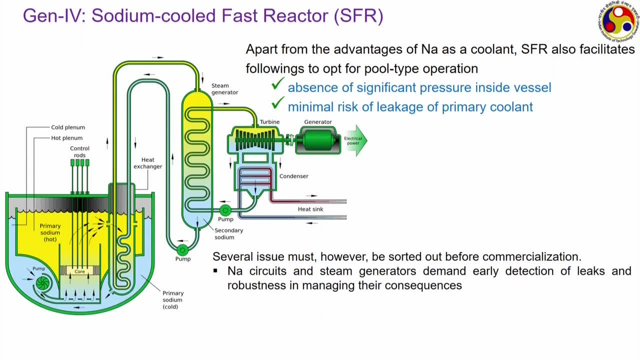 Because even a smallest amount of leak of sodium out of the reactor will bring it in contact with the atmospheric air, which can lead to fire inside the plant. The complexity in in service inspection and repair. sodium is opaque in nature and also we should never allow the sodium to come open to the atmosphere, and that is why in service 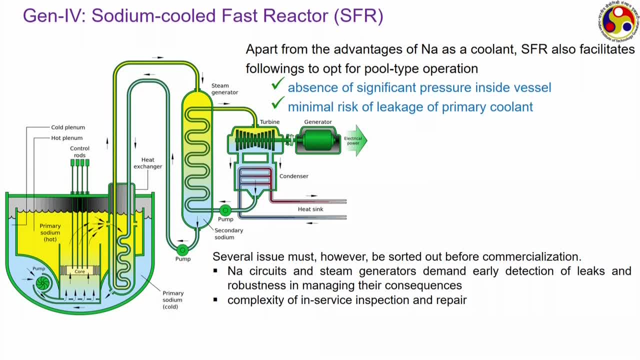 inspection or when the run is going on, the when the reactor is operating. that time any kind of inspection and repair is impossible. SFR can offer an intrinsically positive local void effect As it is using a liquidfuel. if temperature fluctuates inside, then there may be small. 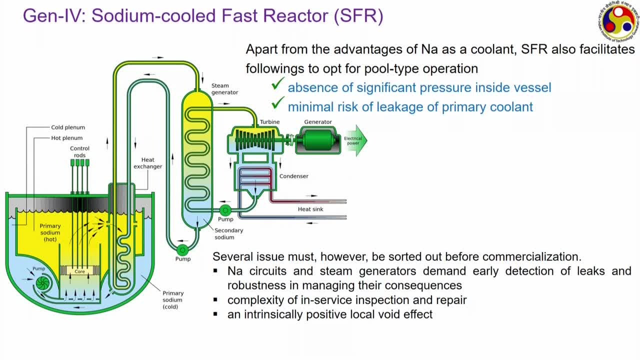 void of sodium appearing or small sodium vapors may start to appear, and if we are having a positive local void effect, then that can lead to a failure of the reactor. So that is something that needs to be Managed generally by optimizing the design of the core and, finally, the improvements. 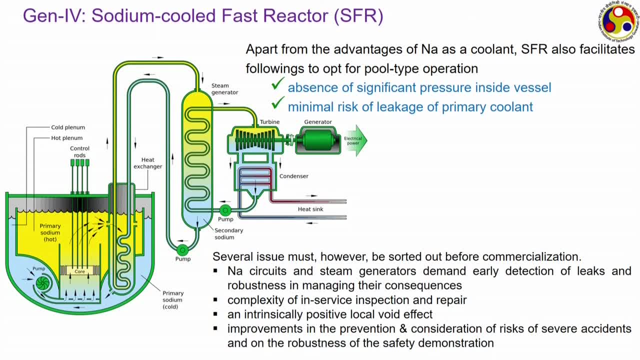 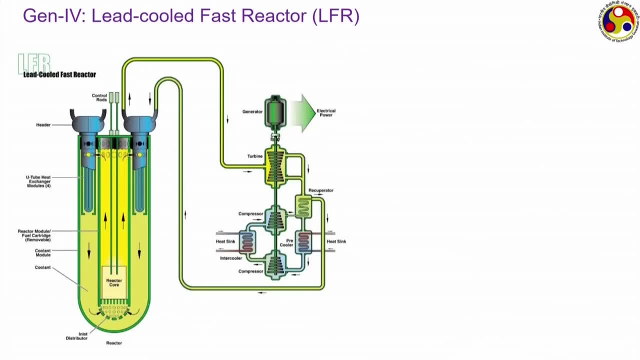 in the prevention and consideration of risk of severe accidents and on the robustness of the safety demonstration, which also needs to be ascertained for this SFR. Next we have the LFR- liquid- or sorry, lead cooled first reactor. The biggest issue with LFR is its highly corrosive nature. Lead has its own advantage over sodium, like I have. 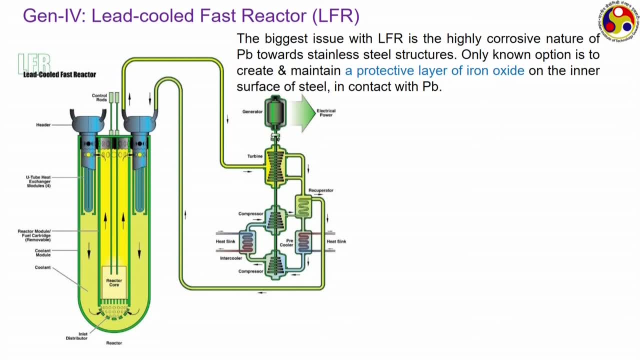 mentioned, It has much higher boiling point and it has a higher heat capacity, but its melting point is also high and it is also corrosive in nature compared to sodium. So sodium lead as a fuel has, or rather as lead as a coolant has- its own advantages and disadvantages, and 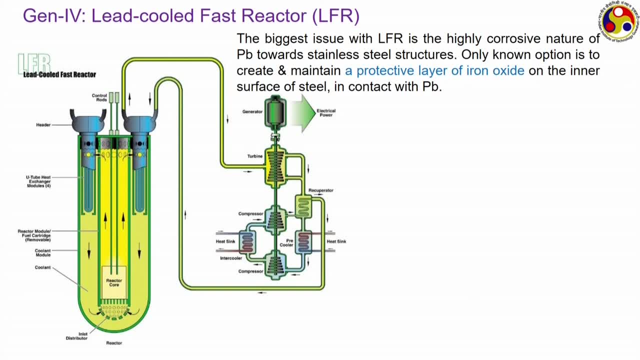 along with that, the LFR itself also. generally, because of the high temperature involvement, we like to use stainless steel as the material and this lead is highly corrosive to stainless steel, which is the biggest issue LFR immediately faces. Only only reasonable option to prevent such kind of corrosion is to use a protective layer. 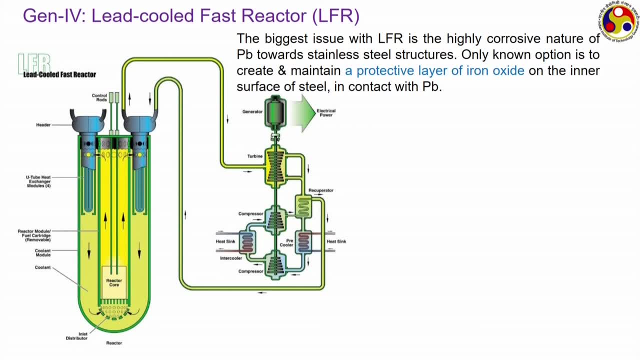 of iron oxide on the inner surface of the stainless steel, The surface which is in contact with lead, that we put a protective layer of iron oxide so that the lead is not coming in contact. So the lead does not come in contact with the steel, but this particular technology. 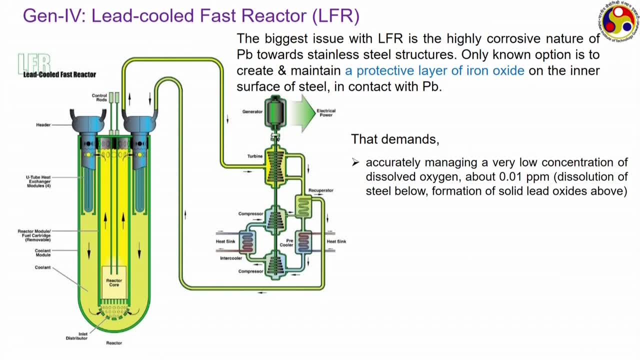 can require quite a few factors like accurately managing a very low concentration of dissolved oxygen, about 0.01 ppm. Maintaining the temperature at every point in the system between 400 and 480 degrees Celsius is quite a narrow band, but we have to maintain this because if the temperature 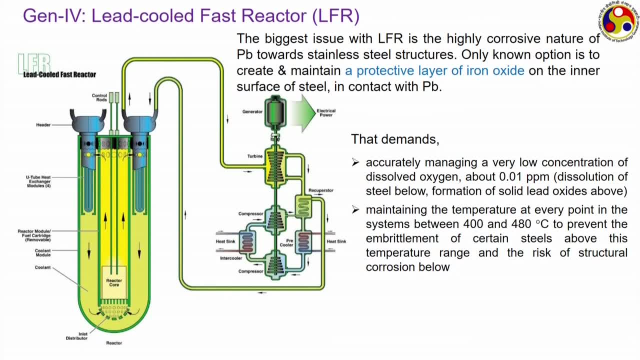 falls this 400 degree Celsius, then there will be risk for structural corrosion, whereas when it goes above 480 degree Celsius, then certain steel may become quite brittle, And also purifying the insoluble lead oxides and corrosion residues present therein. that 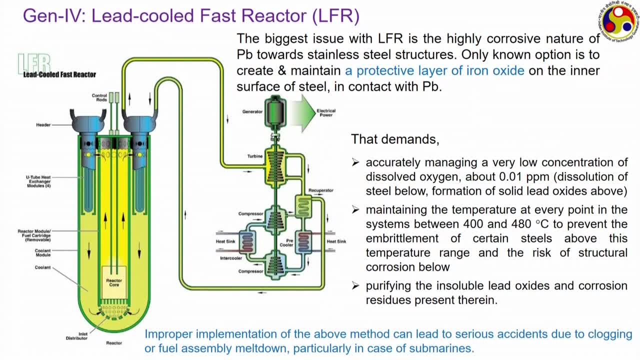 is another thing that we have to consider. If this iron oxide layer cannot properly be implemented, then there can be serious accidents, like those two sub Russian submarines that I mentioned earlier, which are using lead bismuth eutectic kind of material as coolant. 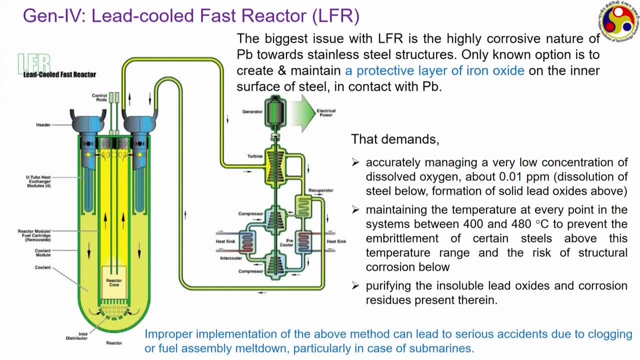 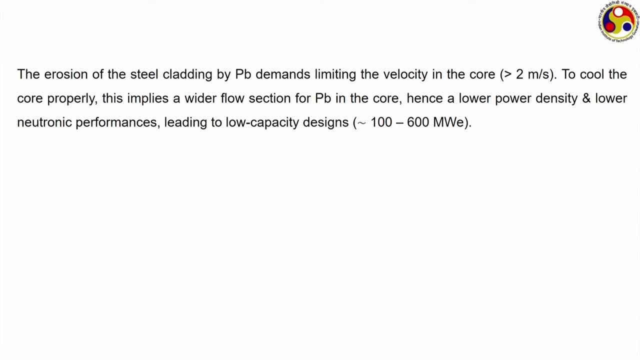 Because of the clogging or fluorescently meltdown, the entire reactor performance of the reactor may get affected. The erosion of the steel cladding by lead can be limited if we keep the velocity small- something less than 2 meter per second. But also if we reduce the velocity, that will reduce the total flow rate of the lead. 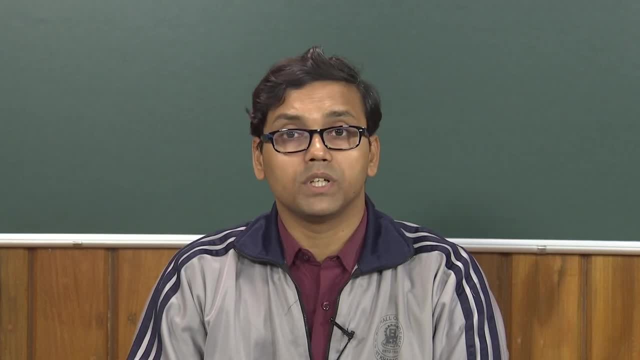 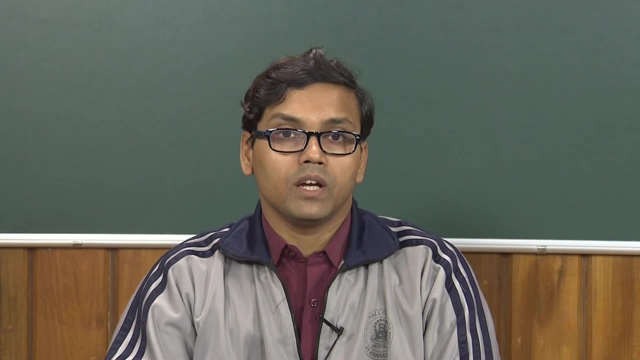 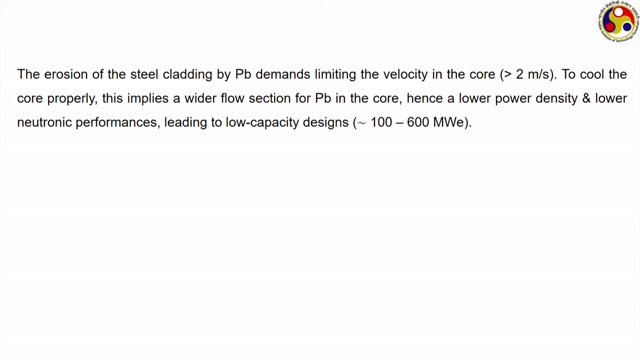 But once the flow rate reduces for a given power output, the temperature rise of lead also will increase across the core, And that will. That is also not desirable And therefore to cool the core properly we need to go for a much wider flow section. 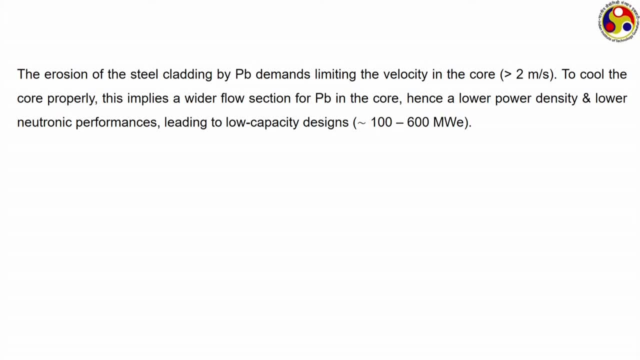 And as they are going for a wider flow section in order to allow the required amount of mass flow rate of lead so that it can take the power output, the total power density, and has a neutrality, performance becomes poor, leading to low capacity designs compared to PWRs and BWRs. 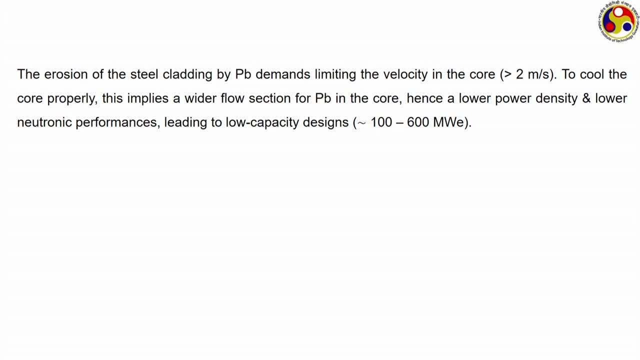 Behavior of molten coal in severe accident situation. that is something that has not been studied at all. The limited database is quite limited And therefore we have to study that, particularly to consider that the lead is much denser compared to both the fuel and steel, which is the cladding material. 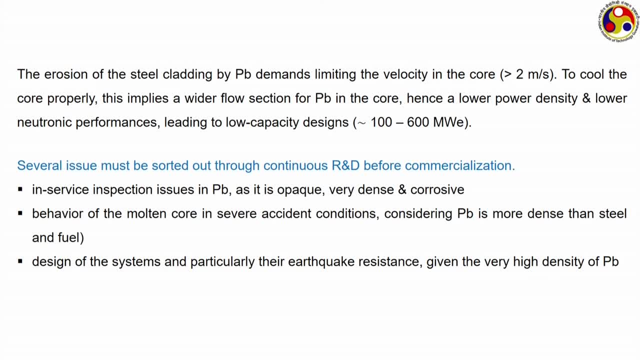 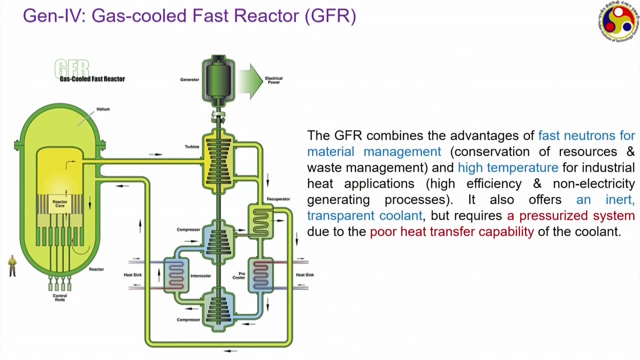 The design of the systems and particularly earthquake resistance, given again, the very high density of lead can be the factor there. And finally, aerosol management, washing and decontamination techniques. It needs to be considered. Finally, the gas cooled reactors, GFR. it combines the advantages of the fast neutron technology. 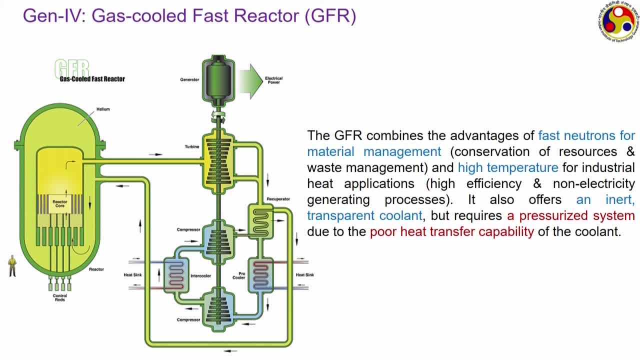 because the material management in fast neutron technology is very high, Resources can be conserved and so is the waste neutrons. Once you are going for fast neutrons, the we can facilitate breeding. Therefore, resources can be conserved. We shall be having much less amount of waste. 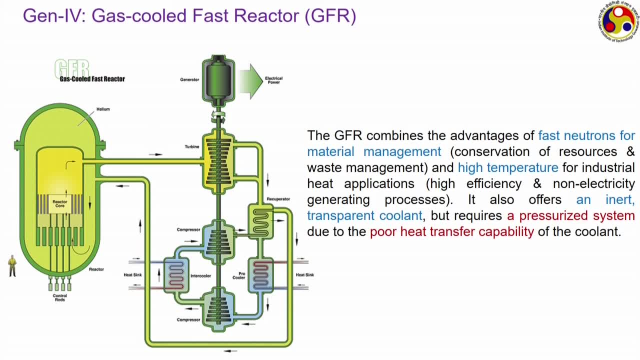 So waste management becomes easy. But also GFR allows to us to go for very high temperatures, As we are using a gas- commonly helium, in certain cases carbon dioxide- as a working medium. we do not need- we never have- to bother about any kind of boiling temperature limit. 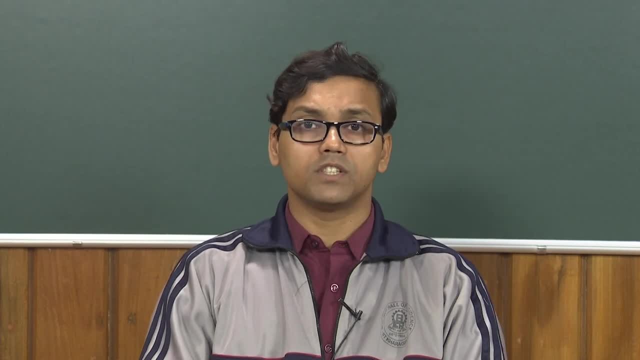 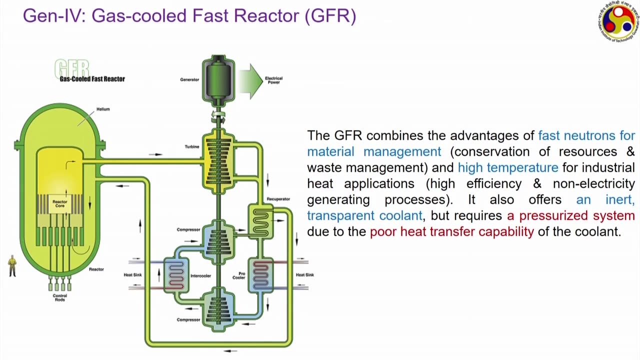 Unless the this, any kind of stability issues or chemical stability issues. at elevated temperatures we can keep on increasing the temperature level, And at high temperature level thermal efficiency keeps on increasing And also non-electricity generating processes can also be facilitated. That is, we can go for some kind of cogeneration as well. 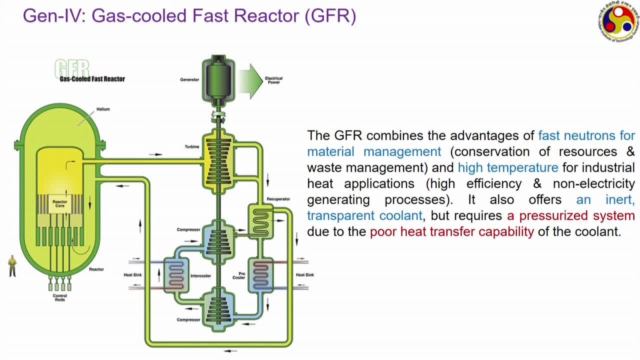 Thank you. Like you can look at this diagram: The hot gas, that hot helium gas that is coming out of this, that generally goes to the turbine And from the turbine it goes to the recuperator and the turbine, after doing the expansion work, it goes to the recuperator and from the recuperator it goes back. 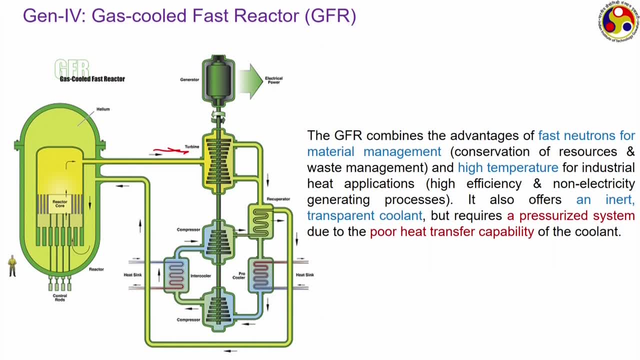 But the gas that we have in this recuperator, or I can say The material or the fluid which is taking the heat in the recuperator, can also be used for other purposes, like such as for cogeneration. And also another advantage: with helium, as the fluid is a, we are having an inert and 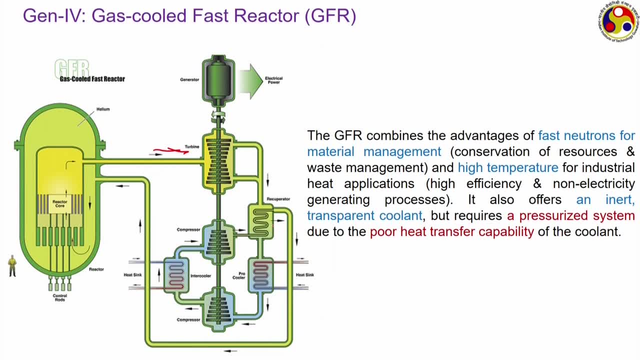 transparent coolant So inside inspection or any kind of maintenance is very easy. It is an inert environment, so no problem with any kind of corrosion or any kind of real chemical reaction when it comes in contact with water or air. But the heat transfer. 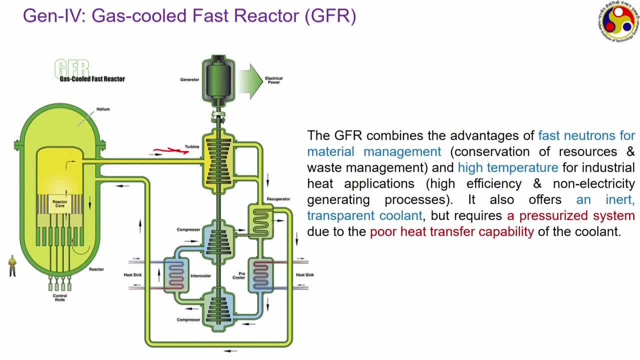 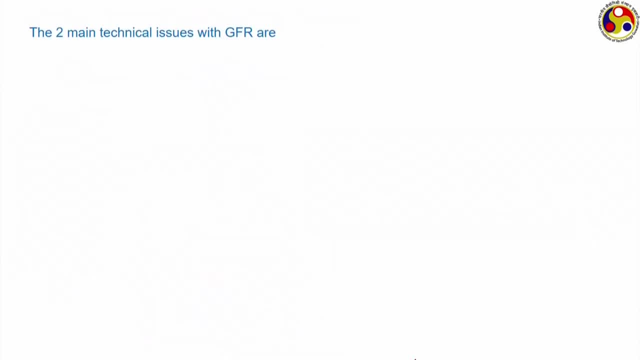 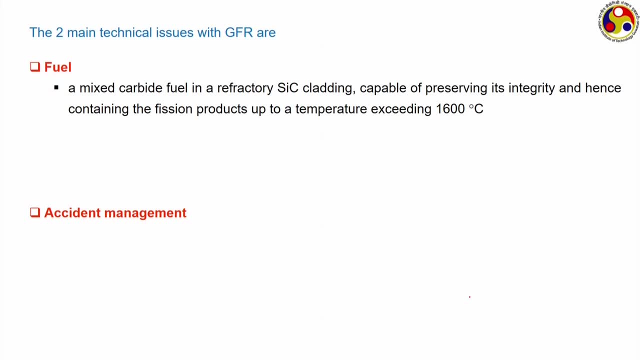 Related to fuel. we need to find a proper mixed carbide fuel which will be put in a silicon carbide cladding and that should be capable of sustaining up to 1600 degree Celsius without any buckling, So that the fission products can be maintained. 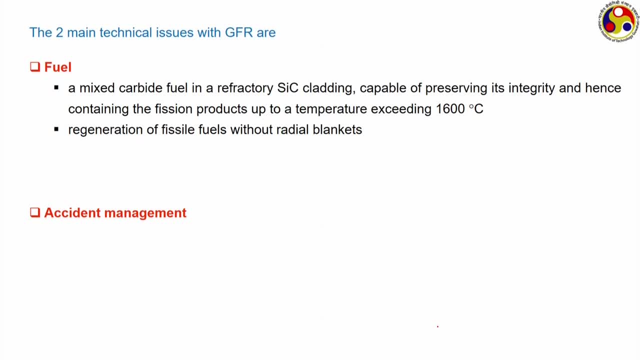 Another is the regeneration of fissile fuels without any kind of radial blankets. And finally is the development and qualification of ceramic cladding which can remain operational for several years, which is not possible with the present day material science, knowledge And with accident management. GFR should demonstrate that the cooling capacity can be maintained. 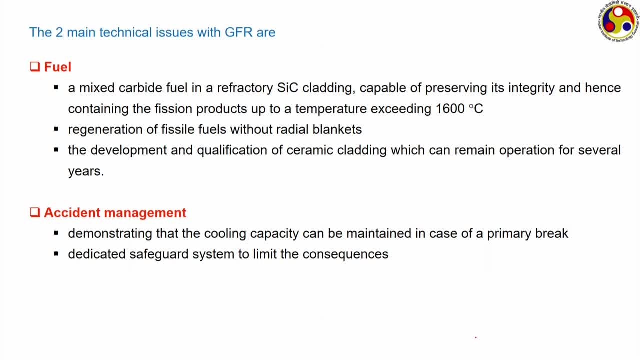 in case of a primary break. Also, dedicated safeguard mechanism is required to limit any kind of consequences of such cooling related accident And also the how the core material is going to behave at very high temperatures are also varying pressure that is unknown, So that is something that also we should look into. 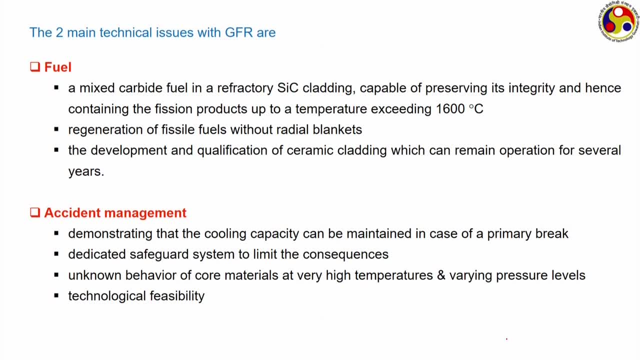 So in and finally, the technological feasibility of GFR should be ascertained before commercialization. So in a nutshell, we can say that all these three first breeder technologies, that is, SFR, LFR and GFR, all of them show immense possibility. 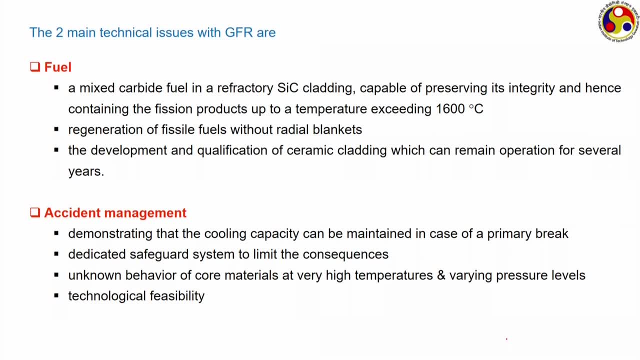 And future And can be the solution for power plant requirement in future. but still there is some way to go because we have to sort out quite a few issues. That brings us towards the end of this module, but I would like to finish with a small numerical. 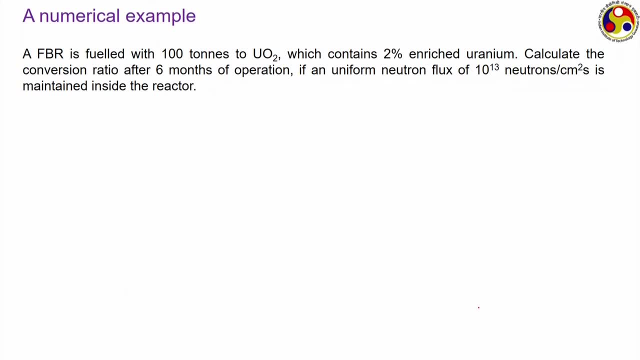 example, related to this breeding ratio. Let us consider we have a breeding reactor which is filled up with uranium oxide as a fuel, a certain quantity of uranium oxide which is has 2 percent of enriched uranium, And you have to calculate the conversion ratio after 6 months of operation if it is subjected to an uniform neutron flask- Now 2 percent. 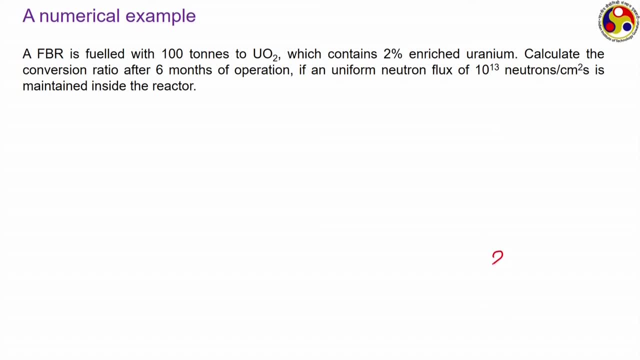 enriched uranium means the fuel contains 2 percent of. sorry, the fuel contains 2 percent U 235 and 98 percent U 235.. U235 will go for fission reaction, thereby produce the fission fragments, and U238 will participate. 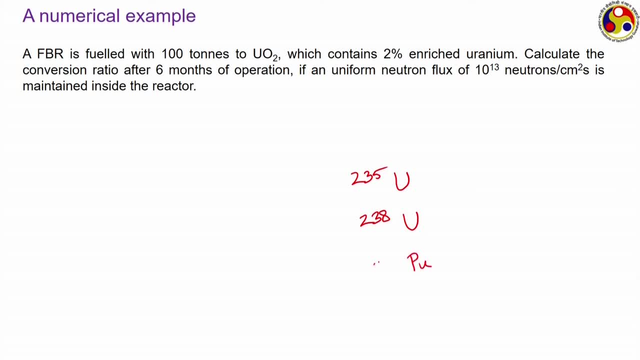 reaction. So as time goes on we shall also be having Pu 239 produced inside the reactor. So initially Pu 239 concentration is 0 to start with, but a time goes on it will keep on increasing, whereas concentration for both U 235 because of fission and U 238 because 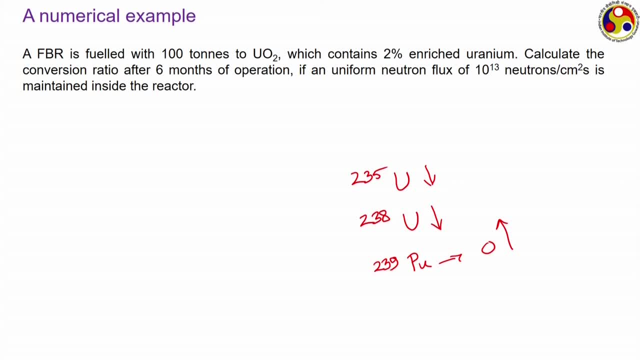 of this breeding reaction will keep on coming down. And actually plutonium concentration, we are not sure that it will continue to keep on increasing, because it will increase because of the breeding but it will also decrease because of its own fission decay. If you just go back to the module number 6, there we made a small mathematics to discuss. 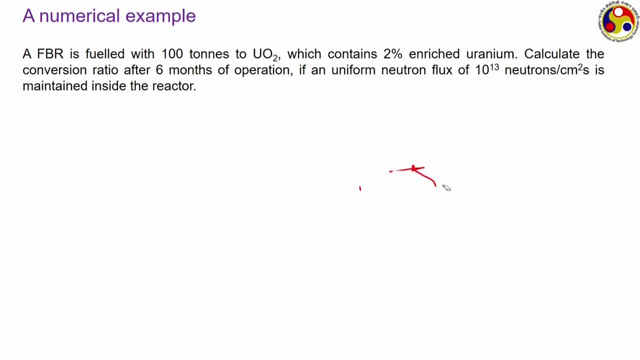 about the control issues, And there we identify this expression. N 25 refers to the concentration of uranium 235 nucleus and how it changes with time, This one beings the H 25.. So this is the concentration of uranium 235 nucleus and how it changes with time. this one being is the 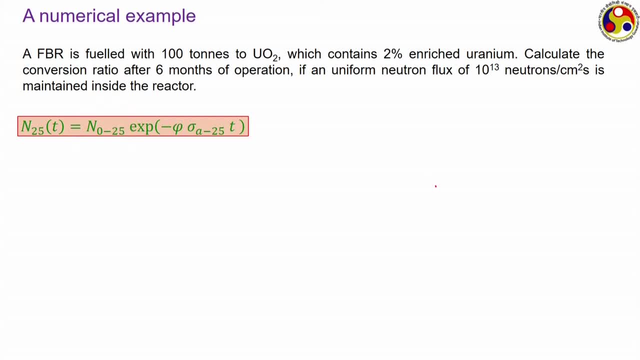 initial concentration. Then N 28 refers to uranium 238 concentration. this is again the initial one. in this case this is 98 percent and plutonium concentration is initially 0. So this N 49 refers to Pu 239 and these are the corresponding cross section values. So 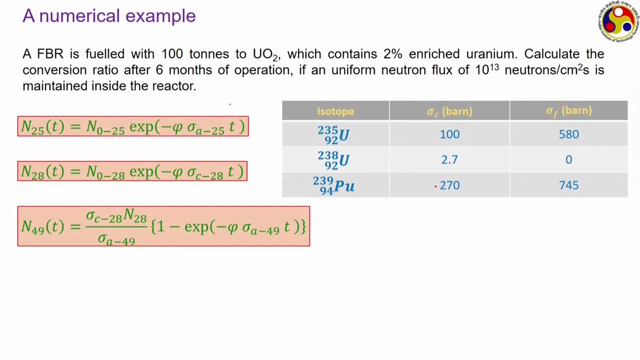 using this, our time period- this t is referred to as 6 months in this case- And, as we already know, the molecular weight or the mass number for all these 3 isotopes. So we can always calculate the value of this N 0, 25 and N 0, 28 and phi and all the sigma. 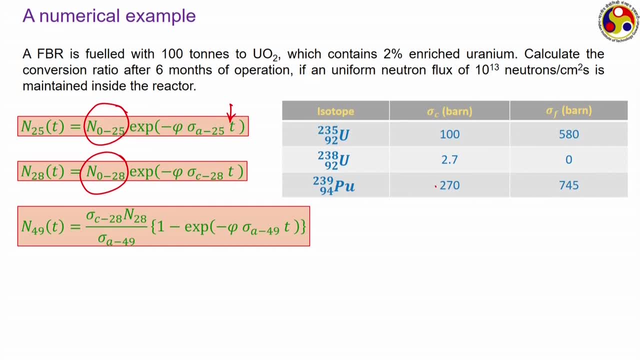 values are given. So at the end of 6 months of operation we can calculate the values of these 3 quantities. And now conversion ratio, at any time, is given to be like this. So using this, you can calculate the conversion ratio, right. 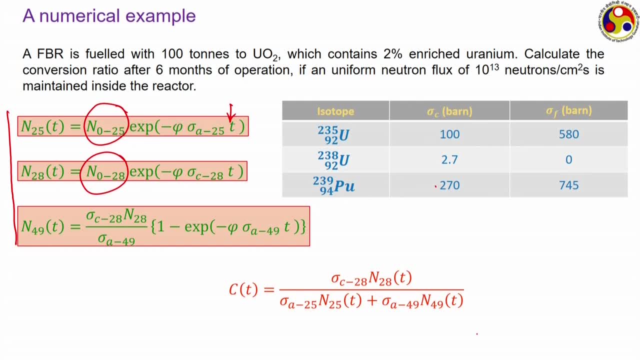 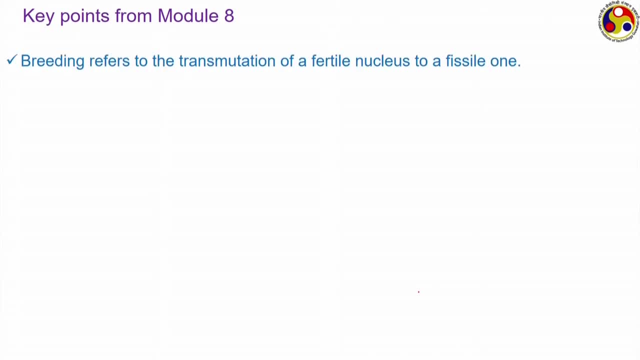 I am leaving this to you. please try to solve this problem and if you face any issue then you can get back to me. So, to summarize our observation from this module, we know now that breeding refers to the transmutation of a fertile nucleus to a fissile one which can act as a fuel for 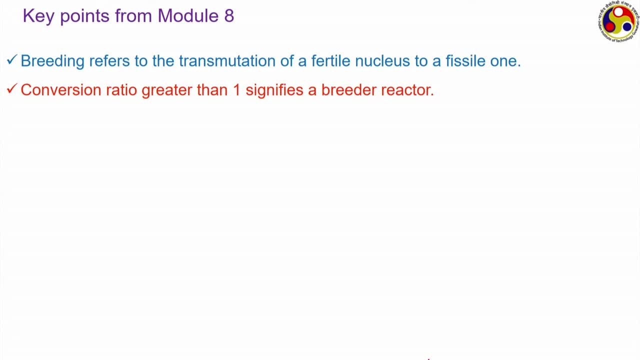 another reactor, or maybe in the same reactor. Conversion ratio greater than 1 signifies a breeder reactor, whereas when it is less than 1 we generally get burners or converters. And doubling time is the time which is required to make that conversion, the conversion time. And the reaction time is given as 0.. So, for instance, I am leaving this to you. please try to solve this problem and if you face any issue, then you can get back to me. And so, to summarize our observation from this module, we know now that breeding refers to the 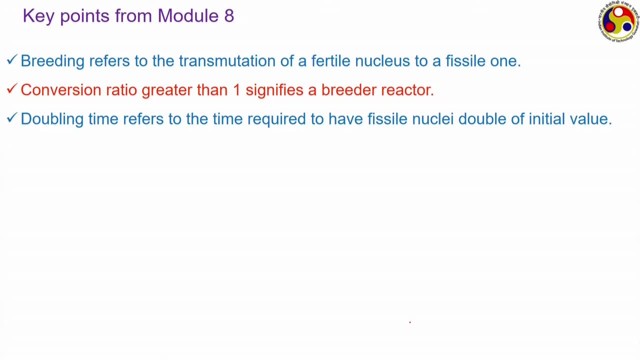 make the number of fissile nucleus double than whatever we had initially. Then we have this, and we have also discussed about the thermal fission factor and temperature, the role they play on deciding this breeding ratio. Then we discussed about the fuel cycle and we have seen that in all the processes generally the mined uranium is converted to. 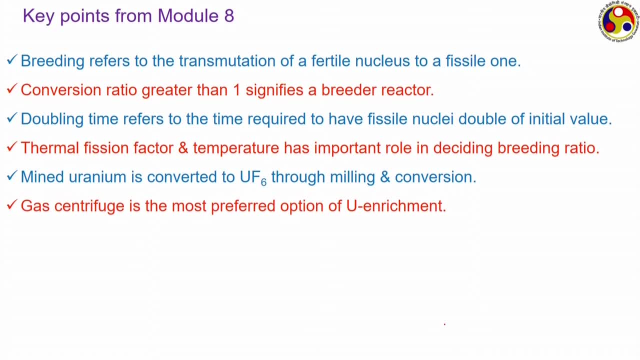 uranium hexafluoride gas through milling and conversion, and then we go for theenrichment process. Gas centrifuge is the most preferred method of uranium enrichment. Then FBR offers much higher power, density and compact designs compared to the thermal reactors, but it requires much superior control. We have discussed in detail about the pros. 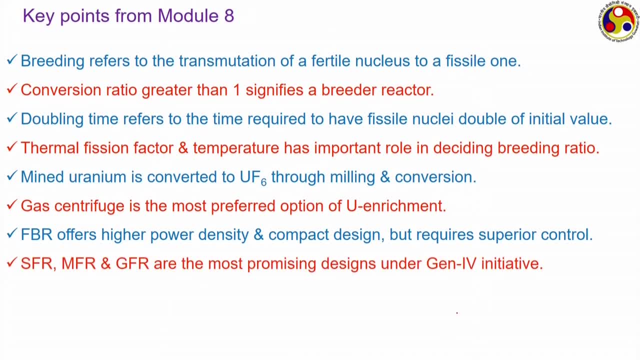 and cons and FBR, and also its comparison with the PWRs or thermal reactors in general: SFR, MFR and GFR. actually, instead of MFR I should not write MFR here, it should be LFR. So we have discussed about the thermal reaction factor. and then we have seen that in all the processes generally, the mined uranium is converted to uranium hexafluoride gas through milling and conversion, and then we go for theenrichment, and then we go for theenrichment. So we have discussed about theenrichment. So we have discussed.